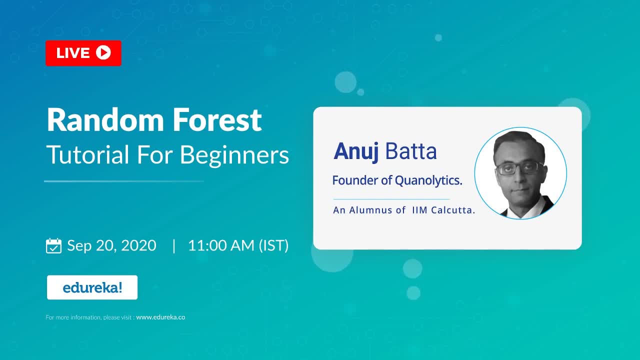 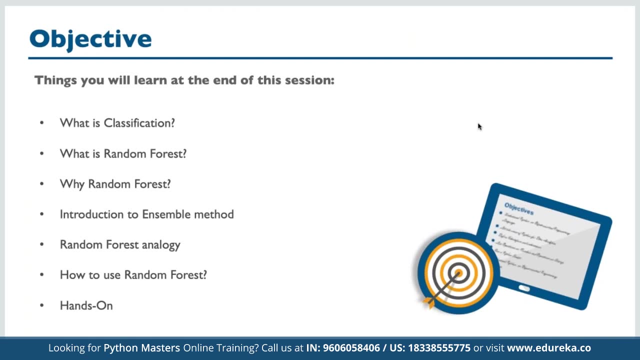 able to bridge the gap between academics and the industry. Today we are going to cover random forest, So we'll talk about classification. What is it? How is it different from regression, et cetera, Different models which we can use? What is the concept of random forest? Why we use it. 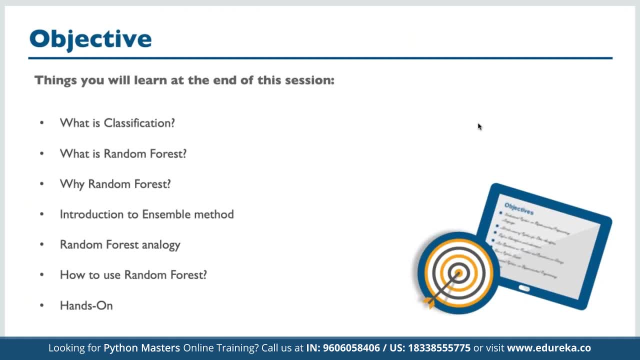 What are the advantages, What are the things which you need to take care of when you are implementing this? And, of course, this is an ensemble model, So we'll talk about ensembling as well- bagging, boosting, et cetera- the concepts which are used for random forest. So we are going. 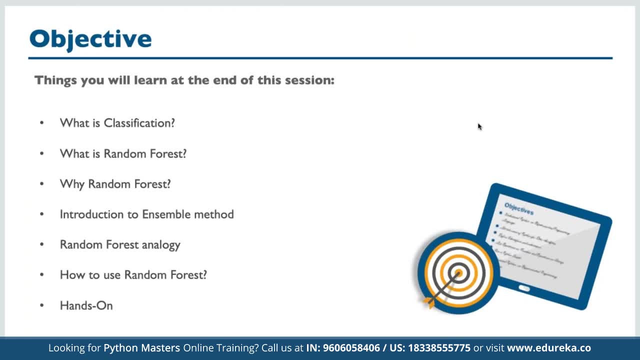 to talk about those. Then we'll give you some analogy to understand why and how we implement this. And then, of course, we'll understand step by step on how do we implement this. And then I'll show you a quick, simple demo in Python so that you also get some idea on how one of the ways to 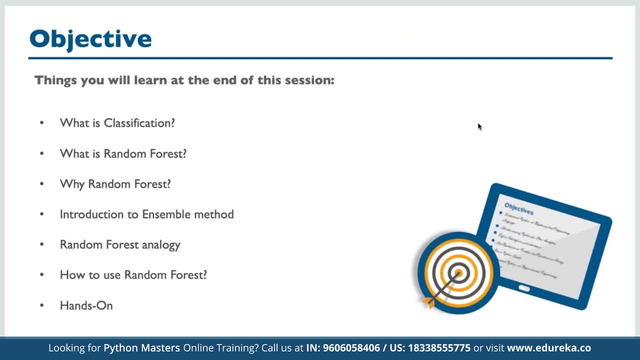 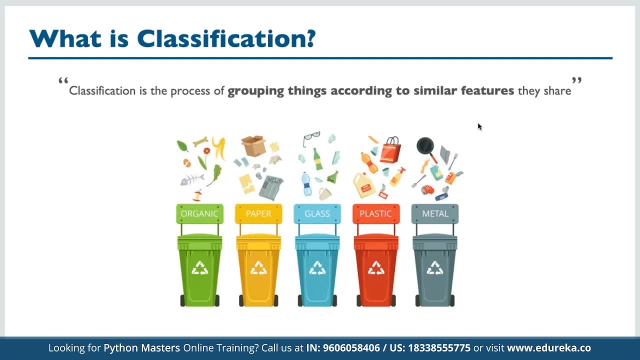 implement random forest. Let's start with the topics. Why are we talking about classification here, Even though random forest can be used for both classification and regression, which I'll talk about. but our focus would be largely on classification using a random forest At a very high level in data science. 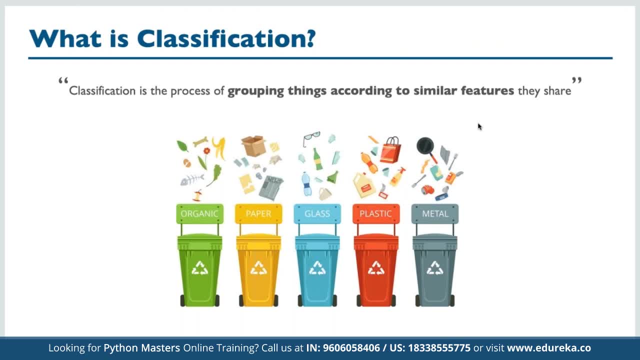 we primarily can do only two things right. We can either do regression, which is predicting a point value, or predicting a continuous variable, or we can put different objects or data points into groups at a very high level. that is called classification. So these are the only two. 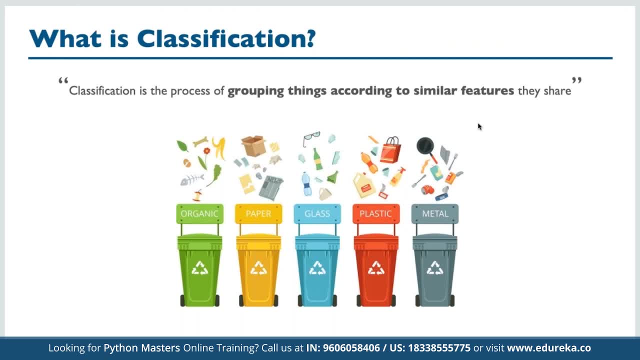 things which we can do. But if we drill down and we look at, you know, further things within grouping of different data points or objects or entities, then we can look at this classification itself as a name, which is a supervised learning algorithm. Or we can also look at clustering, or you know. 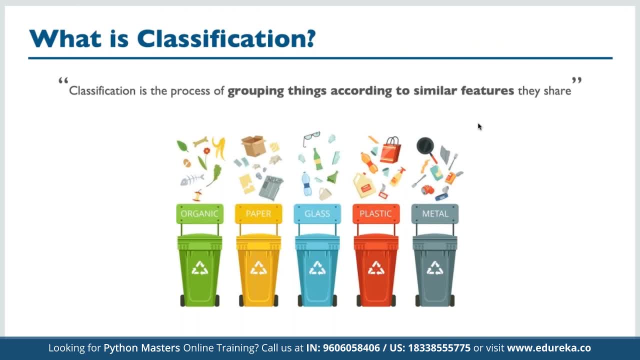 association, mining and things like this, But here we are talking about classification as the specific grouping algorithm. So when we say classification, this is, as you know, good as identifying your data and putting them in some predefined classes. To understand this example, with the image that we 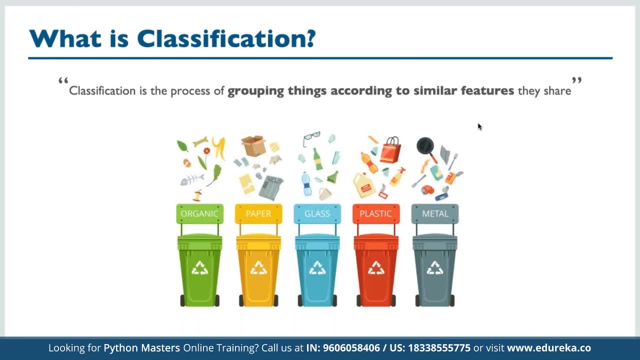 are looking at. we have different trash cans And as human beings we have learned, you know, how to identify different objects and how to map them into different classes. So here we can say this: trash cans which are labeled as organic, paper, glass, etc. 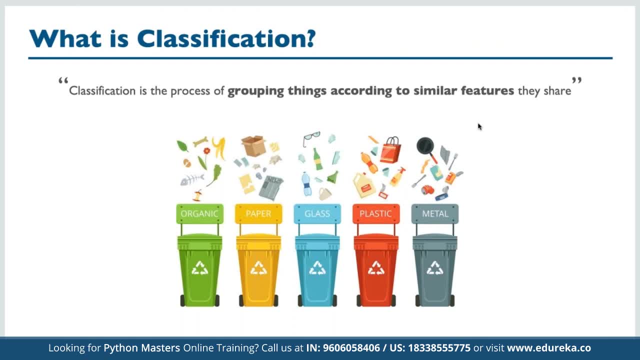 They are different classes or different group names. So why are we calling it supervised learning? Because we know which object would belong to which class. And how do we know that? We have certain mapping done in our brain, based on our historic learning, So we can identify which. 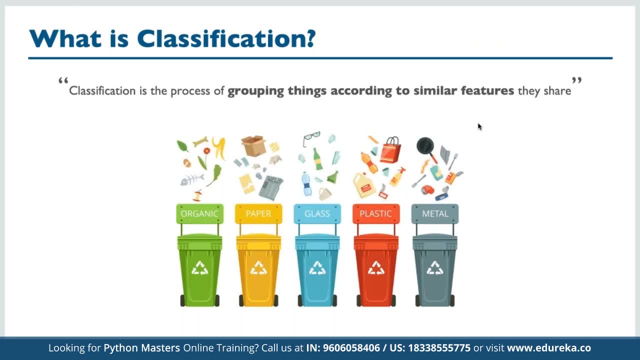 object belongs to which class. right, So we can easily put our waste products into the designated class. And that's what is a way of supervised learning which we also implement in data science. And we are doing classification. So here, every object which is represented here, like fishbone or 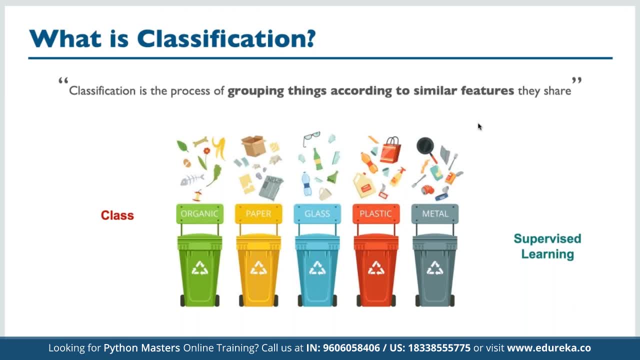 you know, banana or an empty box or things like those are in a data set that becomes a data row If we have to relate this to our data set. so every object which we are looking here and we are trying to put that in a class is actually our data row. So when you get some data set in that, 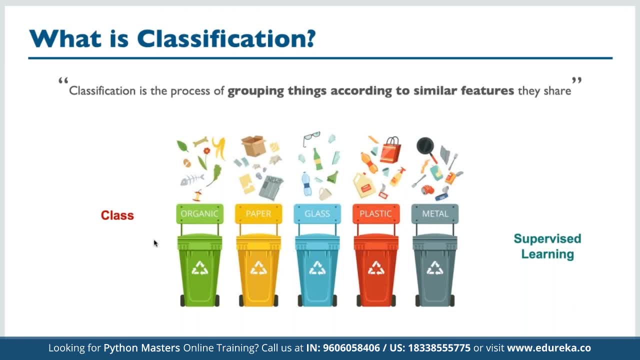 one of the column would be a data class, And all the some data rows individually will represent one object. So what we are going to do is, as human beings, just like we have learned, we will train some of the models which makes most sense in that. 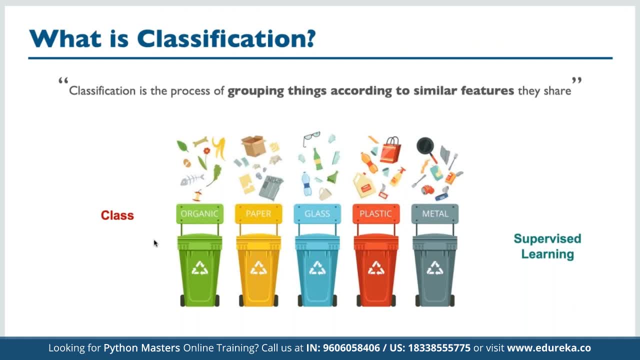 context. We, you know, train that model and we tell that which row belongs to which class. Now, once, on a lot of data, the model is trained, then we can supply with the new row without the class, and the model will be able to predict that which class this object should go into. And that's where we do. 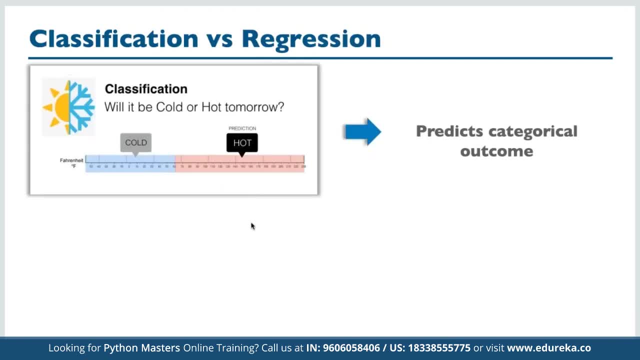 classification using supervised learning. now, as i said, regression means we are doing point value prediction, for example. uh, somebody wants to know what can be the recession in next quarter in my company, right? so that can be a specific value like 9.5 percent or 10.5 percent. so we are talking. 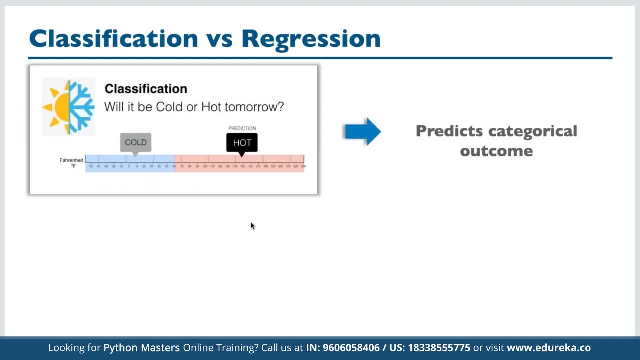 about a continuous variable: how much sales would happen for the new product that we are launching in in uh india, for example? so that is again a point: uh value prediction. so that's what is is a regression. so, if i take this simpler example, when we are trying to classify between uh, we are 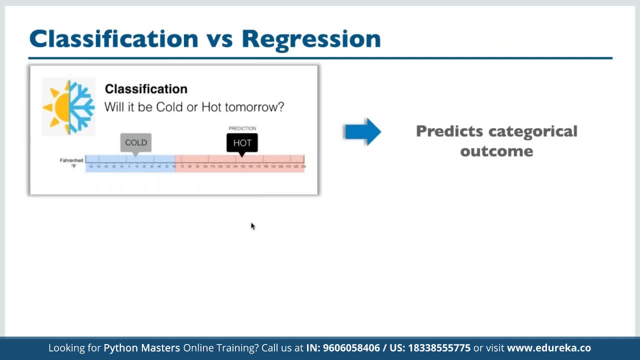 asking a question: will it be hot or cold tomorrow? so we are trying to put uh the data into a class and we have just two classes, so it's a binary classification problem: hot and cold. however, as i said, in regression we are going to predict a a point value prediction. so that's what is a point. 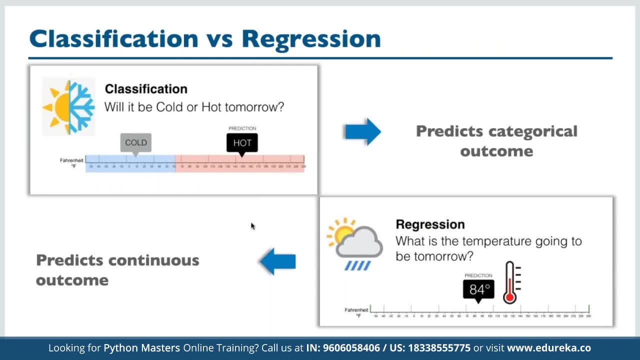 value prediction. so that's what is is a regression. so, if i take this simpler example, when we are trying point value, for example, we are asking a question: what is the temperature going to be tomorrow? right, which would obviously with will be a continuous variable, whether it's fahrenheit. 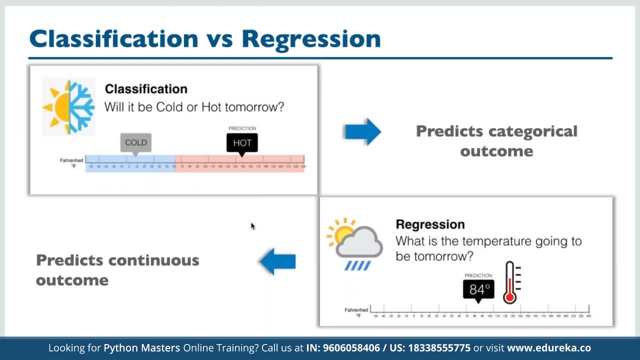 or celsius or uh, you know any other uh prediction which we do, like this is a regression, as i said, uh, there are different models for different objectives. however, there are some models which can be used for both classification and regression, and and random forest is one of those algorithms which can be used for both. now, uh, there are. uh, when we talk about. 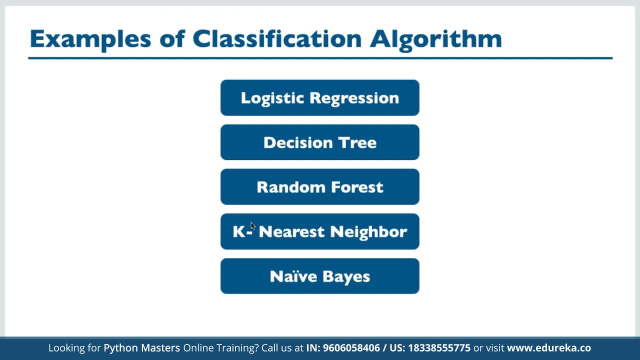 examples of classification algorithms. so i i would also like to point out that, first of all, we should look at the algorithms uh today into three segments, and this is not from the uh regression or classification approach, but from overall uh, uh, you know domain or or the kind of 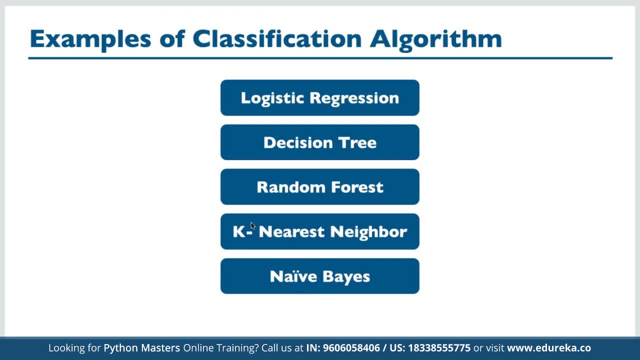 area where which uh, which the uh algorithms are coming from. so we have three set of algorithms generally. first set is of your statistical algorithms, right, which are based on uh, the statistical and mathematical uh equations and and concepts. then we have a different set of algorithms which are bio-inspired or biologically. 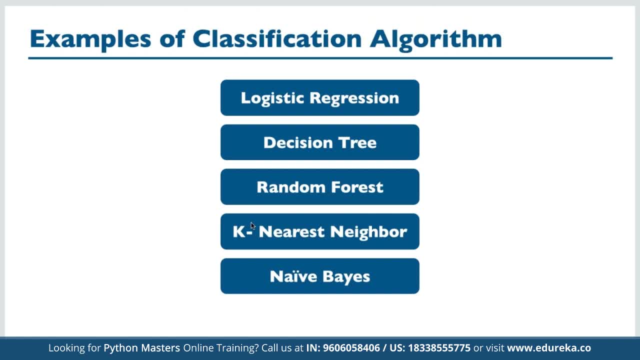 uh inspired algorithms. so you must have uh heard about artificial neural networks, where we try to mimic the? uh behavior of human brain, right? so that's a bio-inspired algorithm, or we have genetic algorithms, uh, as well. then the third set of algorithms are the nature-inspired algorithms, and there are 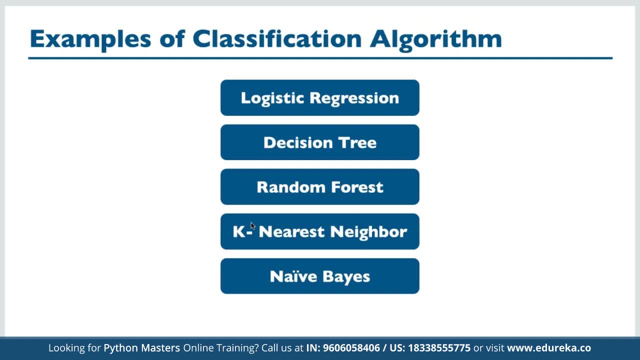 around, uh, at least 100 plus algorithms which are nature inspired. for example, uh, ant colonized algorithm, cuckoo search algorithm, or frog leap algorithm, so, or water ripple algorithm. so what the idea is? uh, whatever happens in nature, uh, for example, if you throw something in the water, there are ripples which are very, uh, you know, in in specific shape and frequency, and 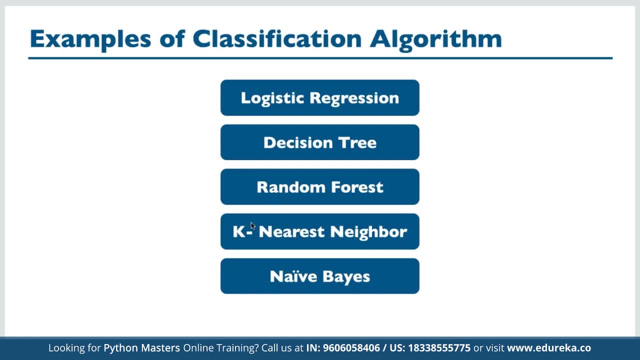 things like those, or when we talk about frog leap. so we know when a frog needs to go from place a to b. it kind of leaps and or jumps, so how does it know that which is the best place for me to jump? uh, so scientists have evolved, you know some algorithms based on this and you know there. 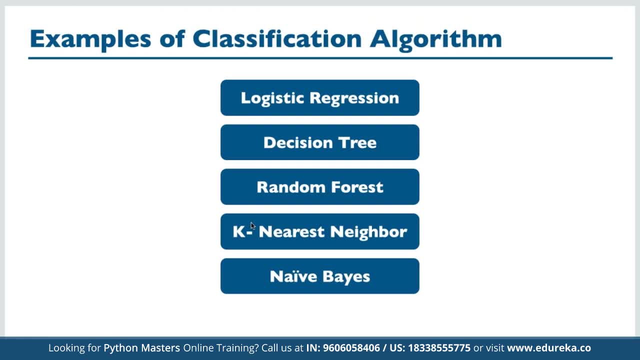 are a lot of optimization problems that get solved due to these algorithms. then cuckoo search again is nature inspired, where the bird cuckoo never creates its own nest. it always puts eggs or lays eggs in somebody else's bird's nest and then it kind of naturally predicts: uh, the highest. 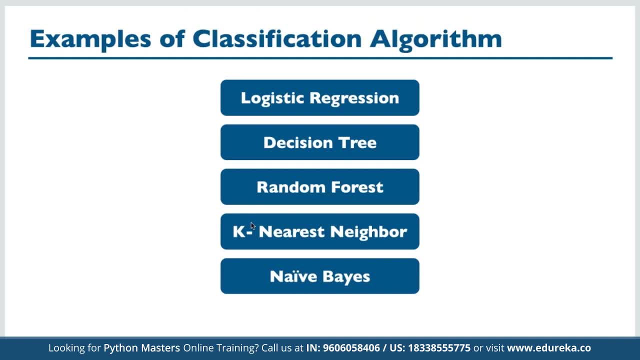 probability where the eggs would be safe and be hatched. so that's where you know, we also try to implement that kind of natural phenomenon and these algorithms, as i said, are widely used. so, for example, uber ola uses this cuckoo search algorithm for one of the 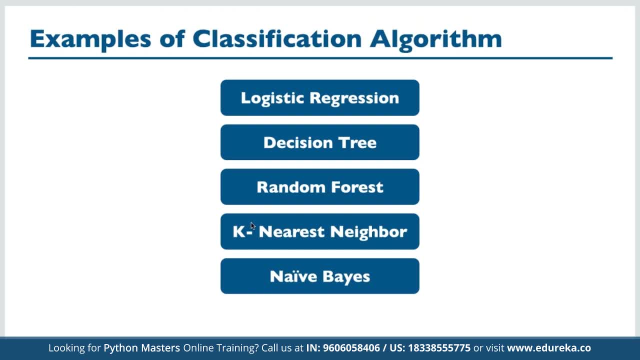 applications when they are assigning caps, etc. so here we are talking about uh, uh classification algorithm and the, the kind of algorithm you look at uh on your on your screen right now. these are the statistical driven algorithms, so we can have logistic regression, decision trees, random forest knife ways, etc. and 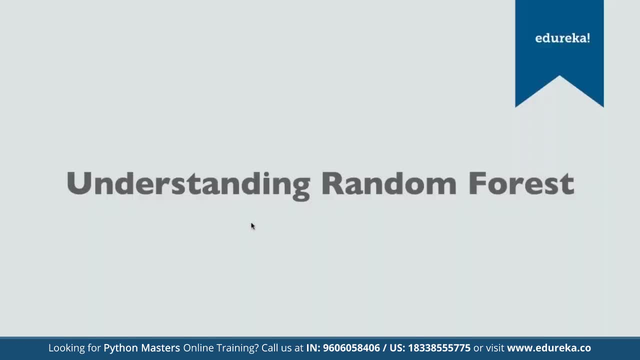 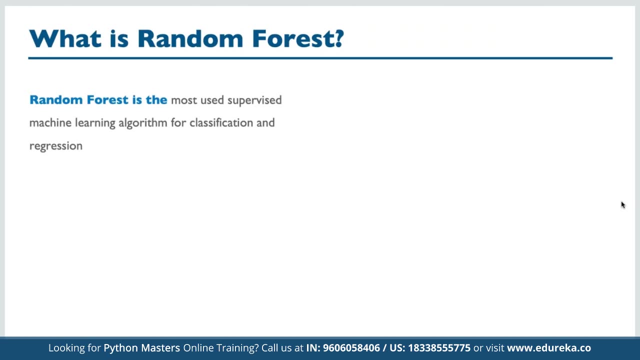 of course, there are a lot more of algorithms in the list. based on the experience, i can tell you that random forest is one of the most widely used supervised machine learning algorithm and, as i said, this is used both for classification and regression. random forests are built on the concept of 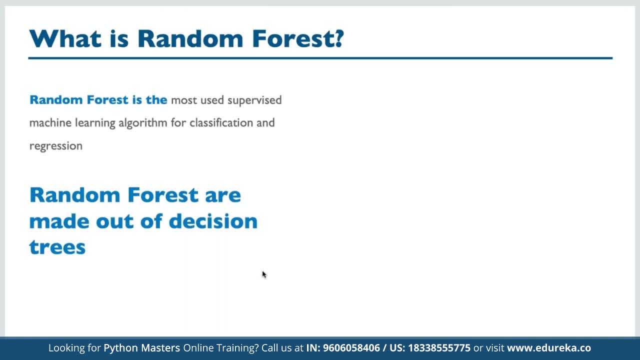 decision trees, and that's where i was saying that it's. it's uh good if you know decision trees already. decision trees are one of the simplest algorithm in terms of implementation, as well as in terms of explaining how things are working behind the scene. right? so decision trees work. 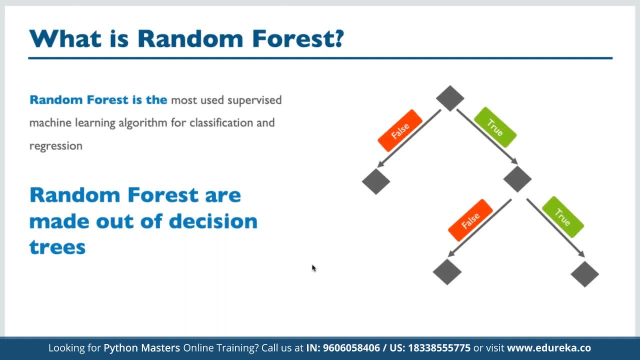 like a flow chart. you start from the root node where you give all your data, the training data set, and based on lot of different parameters like entropy, gd index, uh you know, or other algorithms, it kinds of divide your data set into at least two subsets, as shown here. the data is here the 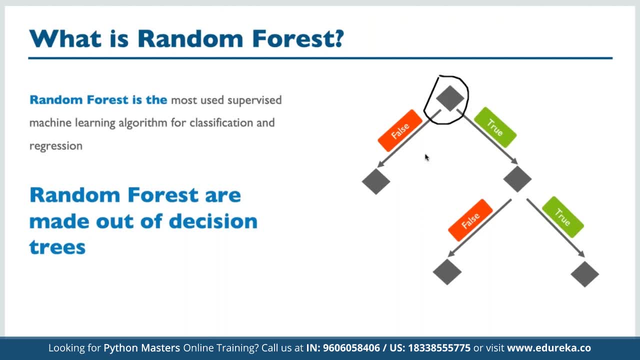 main data set. now it gets. so suppose this is a classification problem. now we are saying the data gets divided into two sets, subsets. one is this, one is this right? so it is subset a and this is subset b. how this data split happens. it happens on different algorithms. 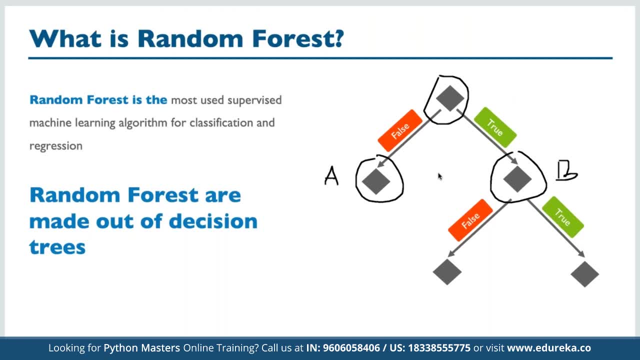 which i am talking about, like genie index, entropy, uh, variance reduction, or there are other algorithms. the primary idea is that we are trying to segment the data so that it gets purer by purer, i mean. the final objective is that all the data should belong to one class. 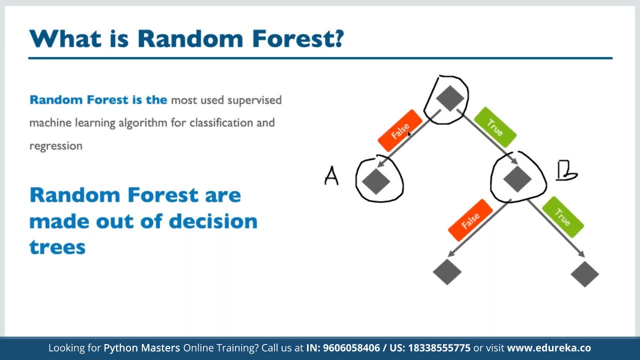 when i have the data on the first node and i have just two classes- false, true and false. of course i have data mixed for both the classes. now i'll run some mathematical uh functions and i will try to divide this data so that i have more uh purity or lesser impurity in a node, which means, if there were, 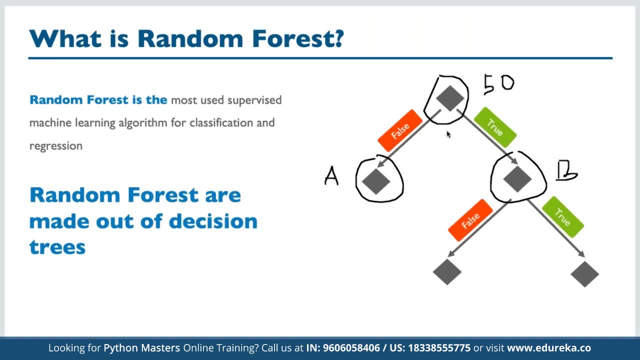 uh, 50 rows of my data out of which say 25 were false, 25 or true. so this is completely impure node. i would try to bring some data where i have false data set is larger here and maybe you know true data set is larger- and i keep on doing this until i get either completely pure nodes or i have some. 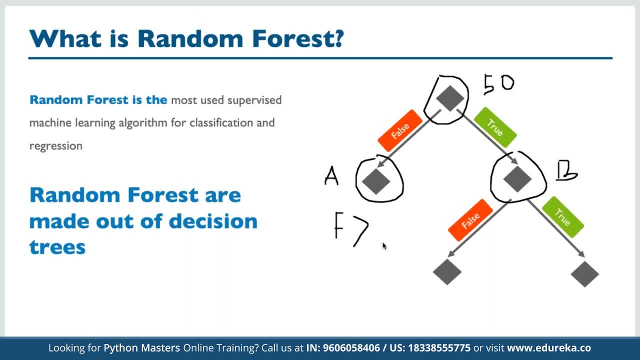 threshold set. so that's a very high level way of understanding how decision trees work. now, as i said, these are the most simplest form of algorithms, because it's very easy to explain to a business user that what is happening, unlike other models which you might have seen, like regression or 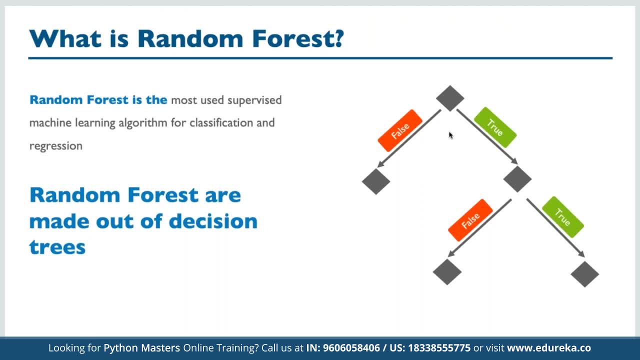 or neural networks or any other model where some mathematics is going behind the scene which is difficult to explain to business users, but here it's very simple to implement and explain. if that is the case, if if decision trees are so helpful and so easy to you know use, then why do we? 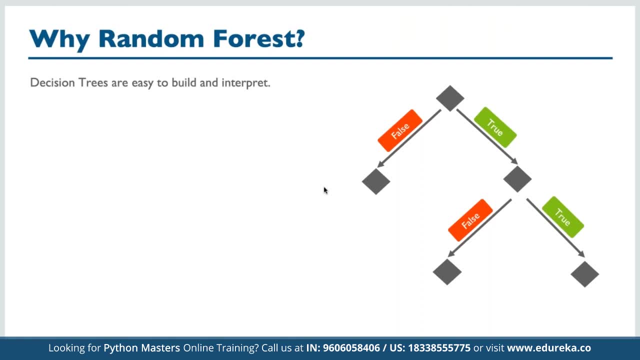 need to uh do something on top of decision trees. so that's what now we have to look at like: why do we need a random forest? so one uh disadvantage of decision tree is that it does not perform very well on the real data set, so it tends to overfit. now overfit is a concept- where it does. 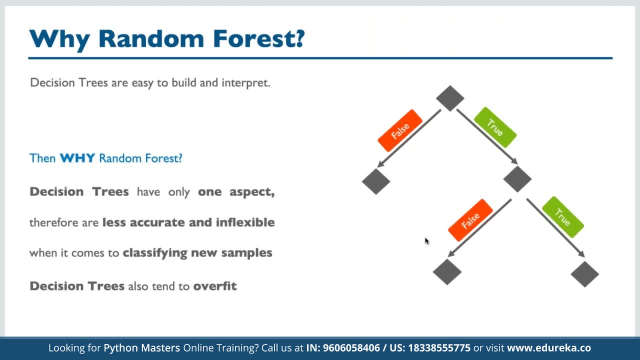 very well on your training data set and it does. it does not do well on your real data, or test data means, uh, you have very high variance. right, it has low decision trees generally have low bias, which is, uh, they, they fit very well on your training data set, but they have very high variance, which 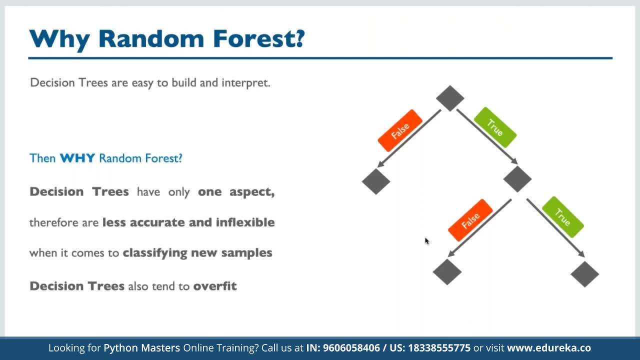 means they don't do well with different data sets, which they haven't seen. to overcome this problem, we still use decision trees, but in a very different form, which is called random forest. okay, so we'll understand what happens. so there's a very beautiful uh uh concept which can help us in understanding. 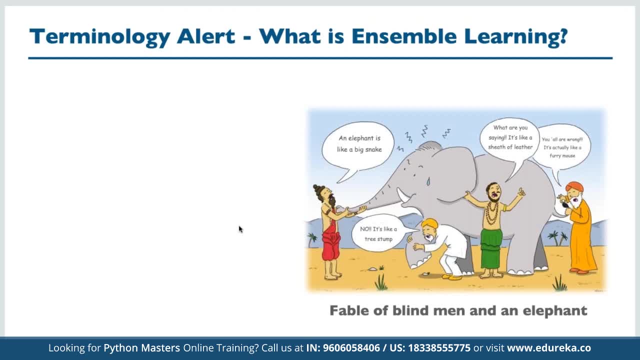 the concept of ensemble learning. so this decision tree is based on ensemble learning. so you must all must have uh read or heard this story in in your uh school days, or you know early childhood uh the family of blind men and elephant. so there are a bunch of uh men who want to know how an elephant 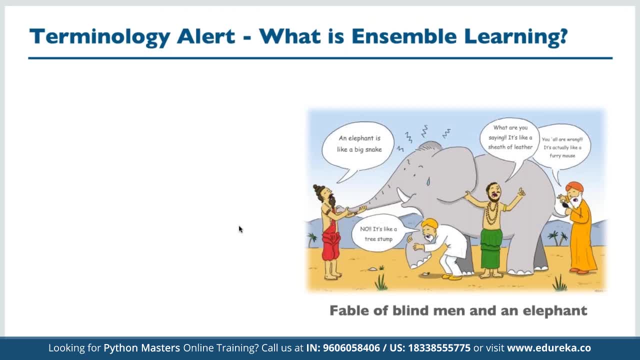 looks like and unfortunately, all of them are blind. so what happens is they try to touch the elephant and try to know how it looks like. so, uh, the person who kind of- uh, you know, touches the trunk, he tells everybody that the elephant is like a, you know, a broad bamboo. somebody touches the elephant from the side and he explains that. 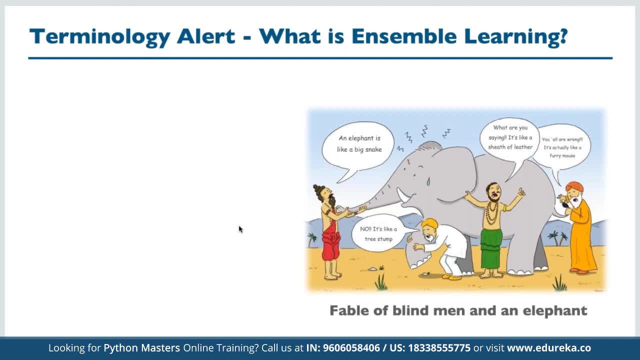 the elephant looks like a wall. somebody attaches his the ear and says it's, it's like a fan. somebody, you know, touches the tail and they say it's, it's. the elephant looks like a rope and they, you know, keep on arguing and and things like this. from this, we, we would understand. 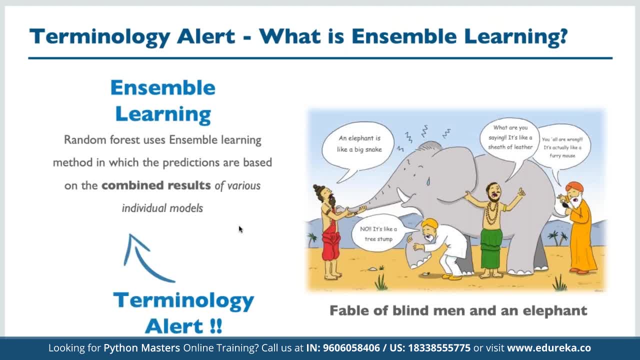 uh, what is ensemble learning? so what happens is when you combine the results based on votes from different uh entities, like it does not use just one model, it uses a lot of different models and then uses a vote to finally identify the class or the prediction value. that kind of approach is called 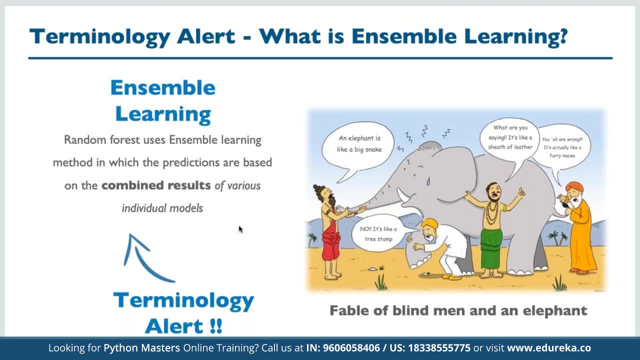 ensemble learning. now, good part about this, versus the story which we have seen, is we can control the data we are showing to different algorithms and this is not something like completely blind people uh checking different uh areas completely of our data set. so there will be a lot of confusion. 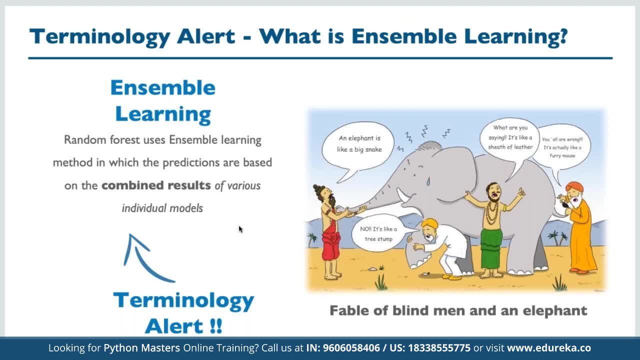 so i will as we'll proceed, we'll understand this in detail that how ensemble learning helps in getting the better predictions than decision trees. but this idea is to just understand that ensemble learning means different algorithms would work on, uh, your data set, in subsets of your data set, and then we'll take, we'll do voting between these two. 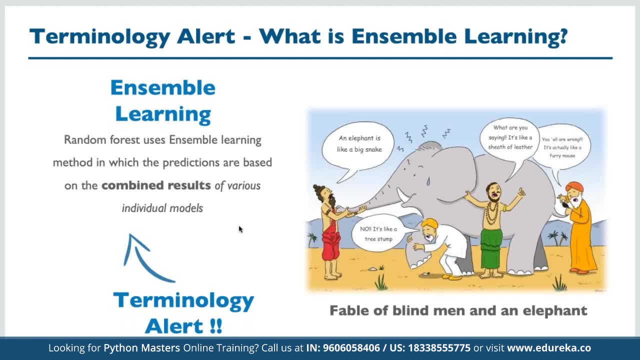 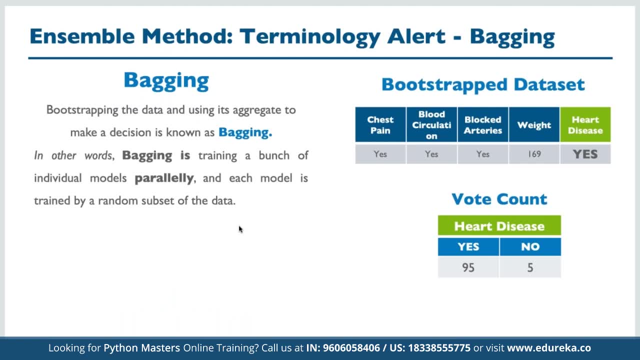 all these algorithms, so there can be like 100 different algorithms which are running under one random forest. so now we'll understand how it happens, okay, so, uh, we will now add. so that was called ensemble learning, so this is a concept. now what we do, what we use in ensemble learning is: 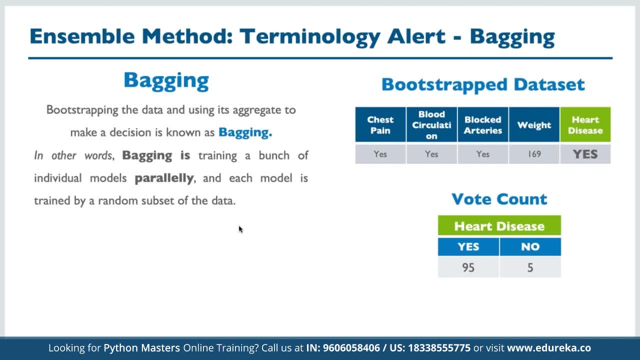 bagging and bootstrapping. what happens is this: concept of voting itself is called bagging. okay, you have a data set and, for simplicity, we are here taking just four variables: uh, chest pain. so somebody is trying to predict whether a a person has heart disease or not based on four attributes: uh, chest pain, blood circulation, some. 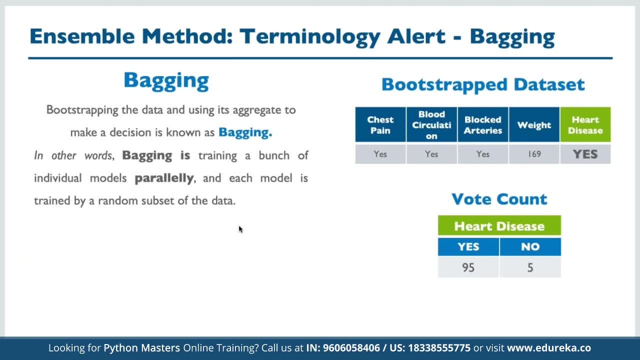 you know, uh, parameter, yes or no, a blog, arteries and then weight of the person. so what we do is we have a lot of data which already has been labeled. so we have a lot of data which already has been labeled. so we have a lot of data which already has been labeled. so we have a lot of data which already has been. 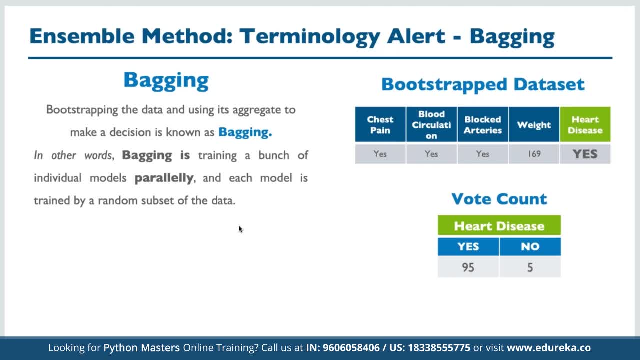 labeled like heart disease is available. so we train the models and then, uh, we take this data, uh take subset of all this data and, you know, train multiple models on top of it. and then, finally, we take word from each module when we pass one specific row. for example, here, suppose we uh, so there were, say, 1000 data rows with these many columns. 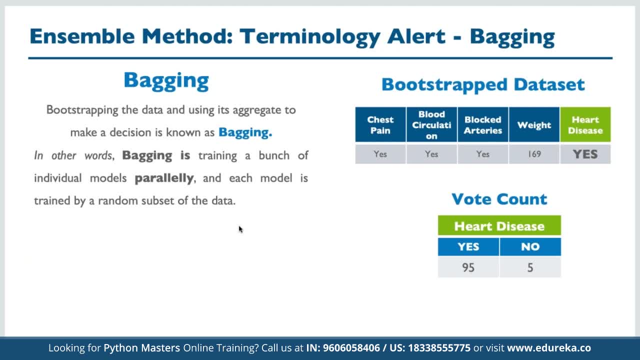 we trained hundred different decision trees or models on this data set and finally we asked every individual t tree that: what do you predict? what should come here, yes or no? and we are saying that, seeing that 95 trees predict the value to be yes for this data which we are passing, yes, yes, yes. 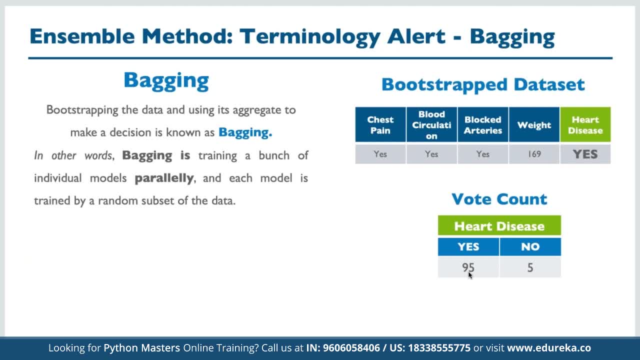 and 169, right? so 95 of the trees are voting for yes and five trees are voting for no, so we'll go with yes, and that's what bagging means, right? so we are running 100 parallel algorithms and then we are aggregating the results based on the votes here. so let's see this in detail. now, what, what? 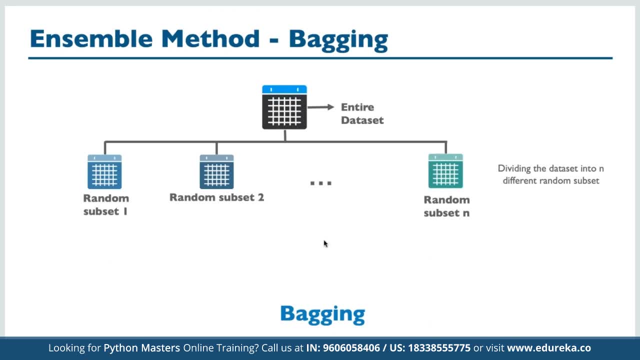 what happens. so you take your entire data set, create n subsets of your data. now interesting thing is: the size of the data remains the same, so all your subsets are equal in terms of number of rows, which means you are taking subsets on random selection with replacement, and i'll explain that. 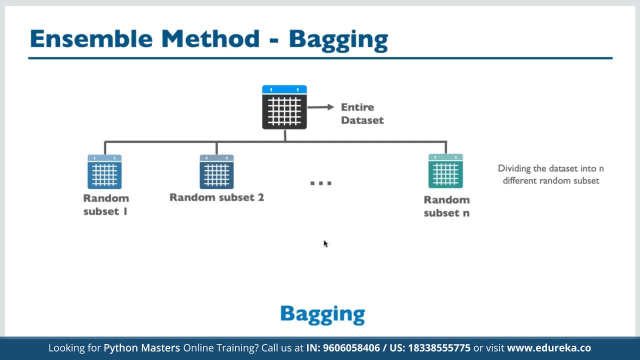 in in the next figure. but just remember that we are creating n. subsets like n can be 100, 250 or whatever number which makes sense. so those many subsets of your data, but all of the subsets have equal number of rows as your main data set. then what you do is you create one individual tree. 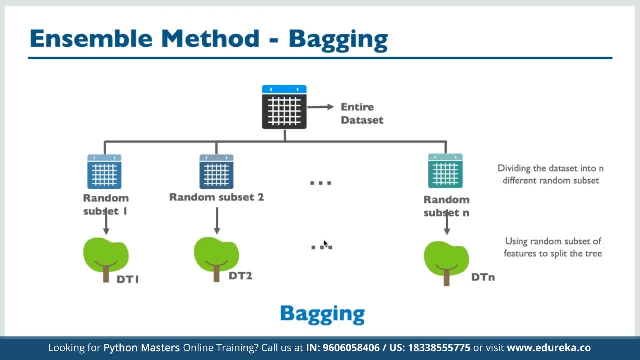 on each data set. now, what is the difference between these trees? one is they are getting same different data because, even though the size is same, but there would be a lot of repetition of rows and then two subsets will not be same or equal to each other in terms of the data. 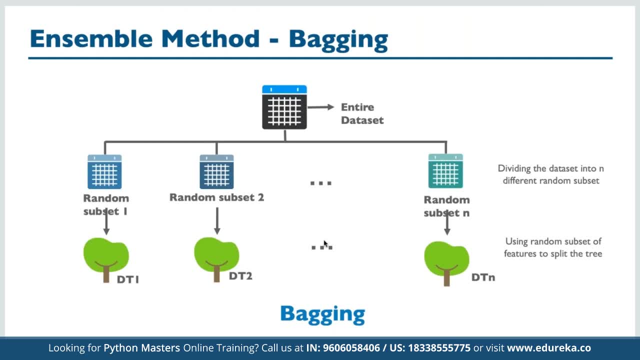 they are same in data count, but they are not the same data. other difference is that every tree is not exposed to all the columns. so if there were 10 columns in your data set, subsets will also have 10 columns, for example, but the decision tree will not be supplied with. 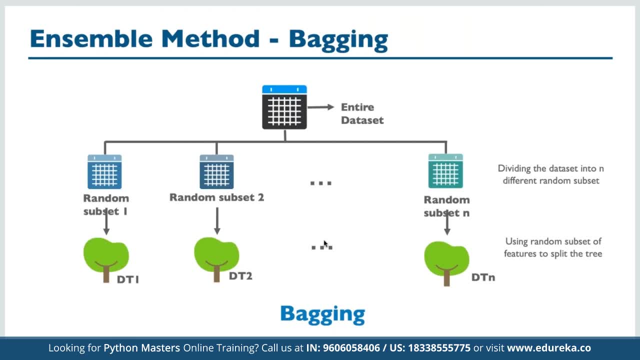 10 columns. they would decide how many columns do we want to give. it give to every node while splitting. it can be two, three, four, whatever number we think is right, and then the tree would be predicting, based on different columns and different data rows. after which we are going to test, and i'll explain how do we do this process in detail. how do we? 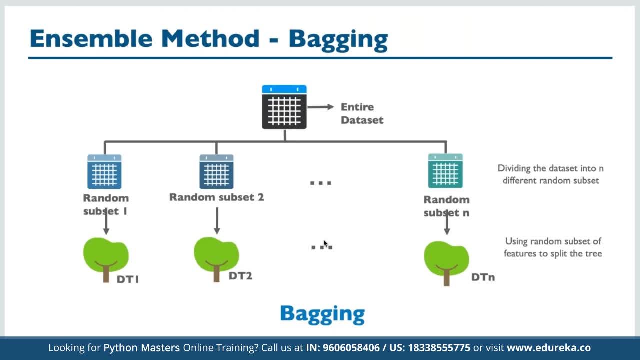 create these data sets and how do we decide how many columns and which columns to pick? but this is the general idea of bagging in. uh, random for us, right? so just to reiterate: take the entire data set, create n subsets of same size. of course data is different, because what we 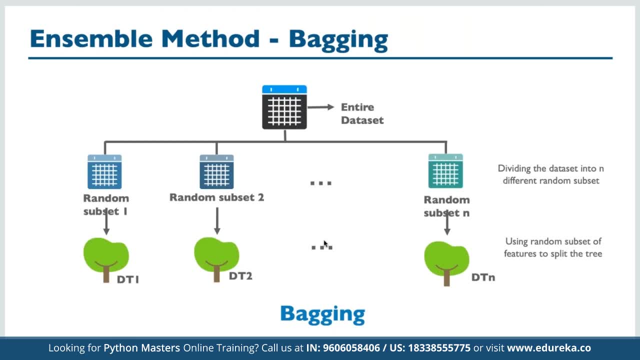 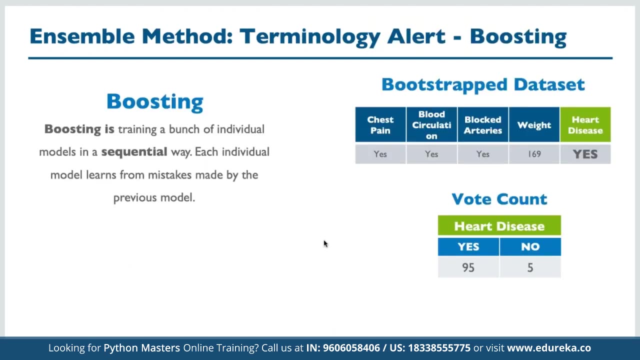 are doing is random sampling with replacement. then we pass on this data to different trees, where we have different columns for the tree and which is at random, and then we are going to train these individual trees and then we take the vote of these trees, as we have something called bagging. 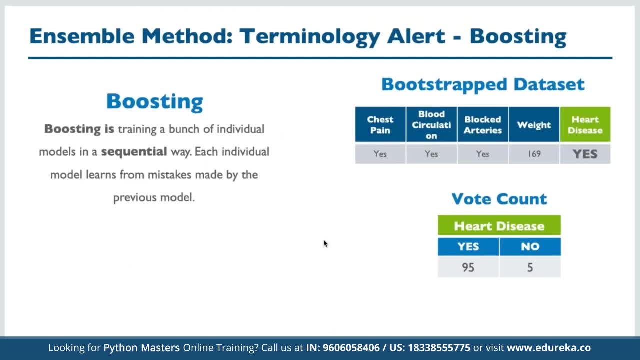 There is another concept called boosting for ensemble learning. but in boosting we do not run parallel algorithms, We run sequential algorithms and there are different algorithms, for this random Forest does not work on boosting- Okay, it works on a bagging. So in boosting, what we do is we take the data set. 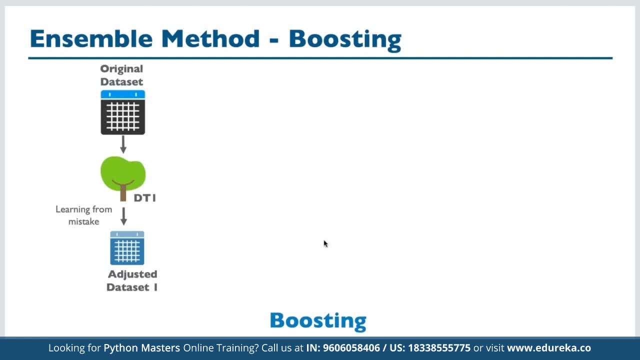 We train one model, we learn from this model, We change a few things, We change some data, We know wherever we have the Max confidence and there are other other things which which happen. then we train the next model, then we get the output. We learn from this, then we train another model. 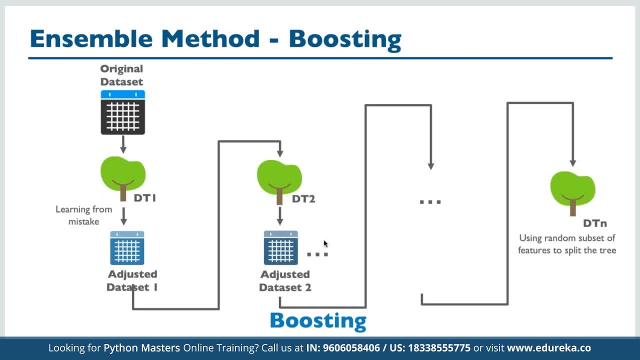 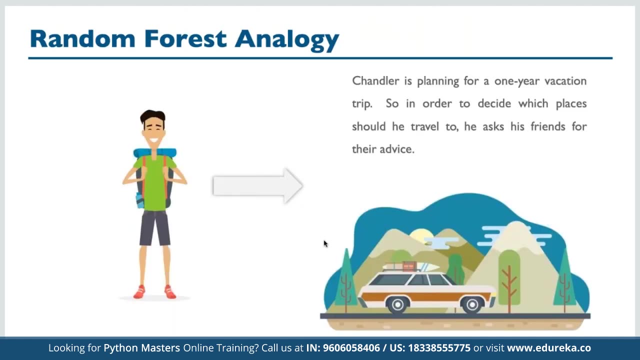 So even here we are using multiple algorithms and models, but we are doing that in sequence rather than in parallel, and eventually we'll have a final outcome. So this is the concept of boosting both bagging and boosting our assembling algorithms. So let's now understand some analogy. 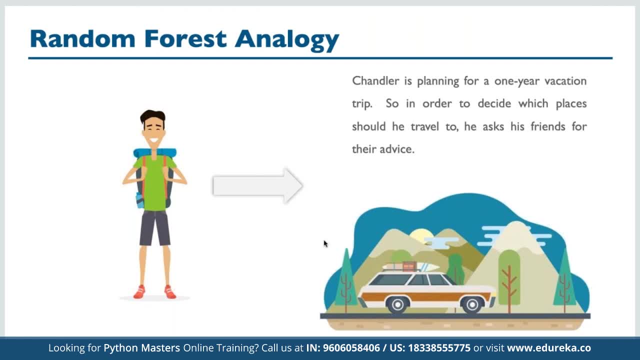 so that we get more clarity on this. So, Chandler, here our friend is trying to plan a one-year vacation trip. Now he wants to choose that- where should he spend his time, and you know things like those. so he's trying to get the destination for his vacation. 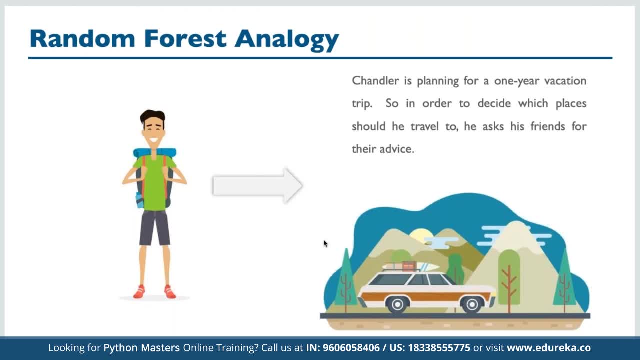 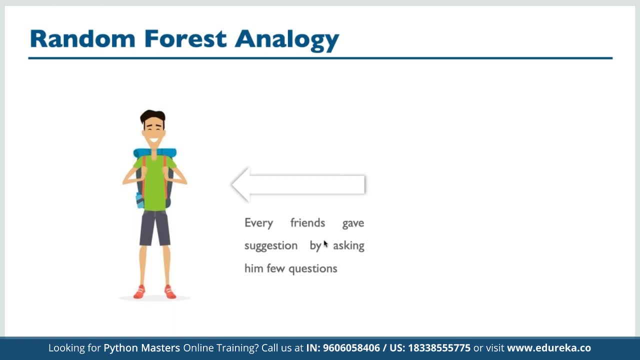 So what he does is he asks a few friends that you know, where should I go now? the friends would ask him questions like: which place do you, would you like to spend time, Are you adventurous, You want to go to calmer place, or things like those. 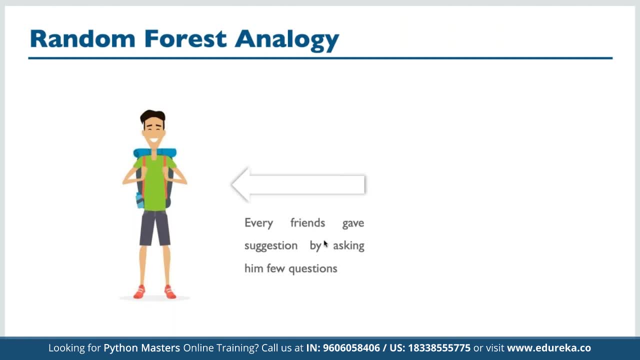 So there would be a lot of questions and I'm asking- I'm explaining this because that's what the tree also do with the data right. So one friend can suggest a specific location, second friend And can suggest another location, third preference, would you know? 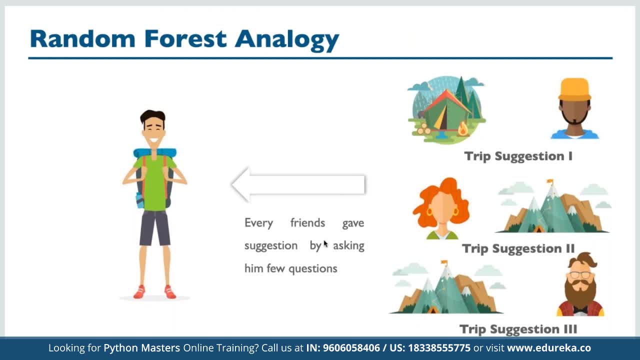 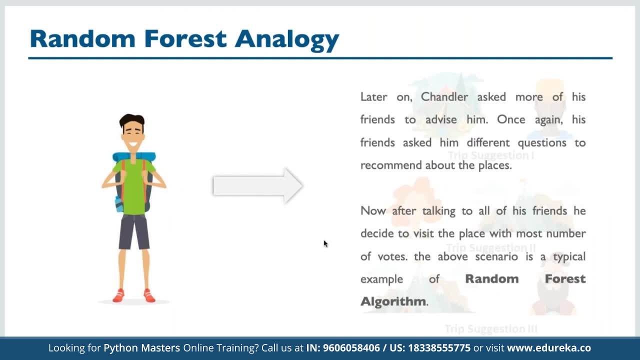 suggest something else and of course there would be some overlap. and then it the process continues. Chandler keeps on asking more friends and you know eventually what happens is, after asking everybody, he sees that what is based on my interest, which place is being suggested by my friends maximum number of times, right? 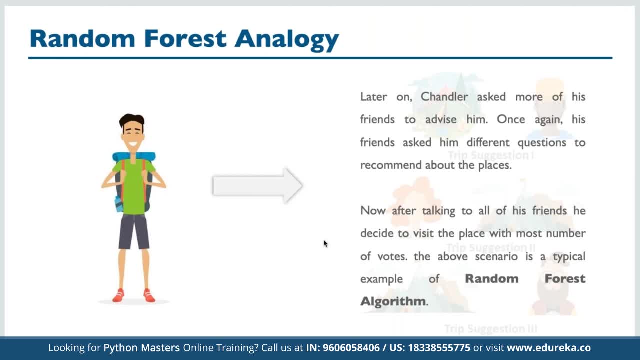 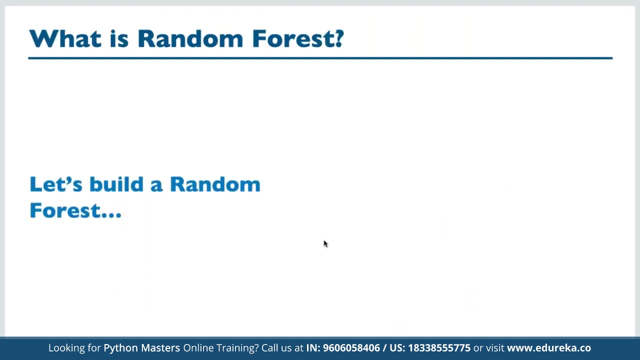 It is just like voting, And that is how your random Forest also work. So you provide information to different algorithms, which are friends in this analogy, and then you finally decide on the maximum number of replies which we are calling as weights. So now, quickly, what we are going to do is we'll again intuitively see. 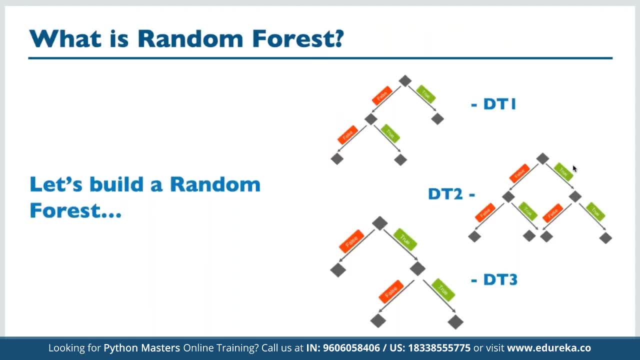 so what we are saying? we have data set. now we are building multiple decision trees, So there will be a lot of decision trees. here We are just showing three. but if you have like 10 variables in your data set and few hundred rows, 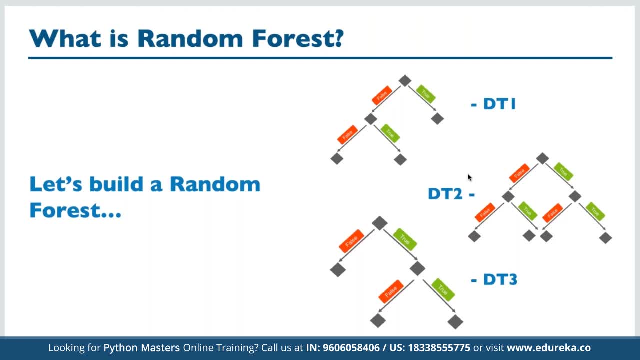 we can easily build, say, 30, 40 decision trees. as the size of data set increases and as the columns increase, you can continue to increase the decision trees, and this all will come when we do the matrix evolution and we see. you know what, what number of trees are giving you the kind? 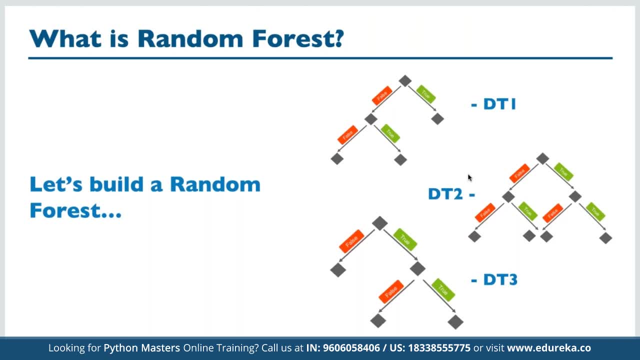 of right prediction. So that's where we decide on number of trees, but we can start from a number based on the suggestions or suggestive measures which are there. So there are no hard and fast rules. as I said, that you know, you always start with 20 trees or 25 trees. 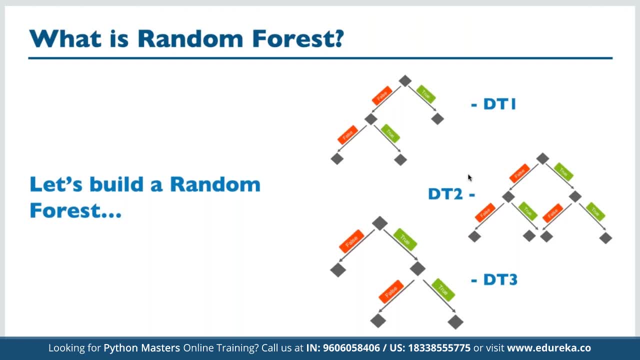 So that's a generic question which is there when you start on this, that where do you start from? so it comes generally with with practice and here it will try, and then, of course, you can get some recommendations from different sources, like research papers etc. This is what looked at. 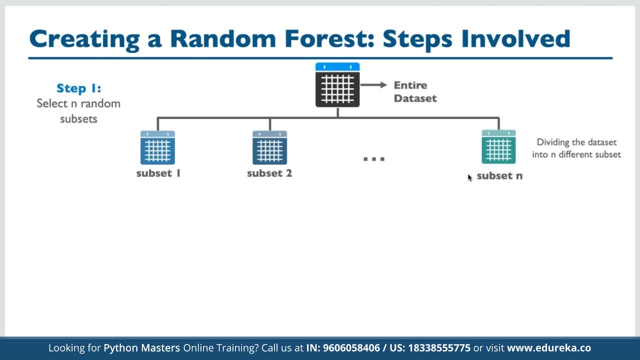 But now we are saying, talking about all the steps, So you have your entire data set. you have divided this data set into subsets. We have the same number of rows, but the rows are not same right. So the we don't have the same data in different sets. 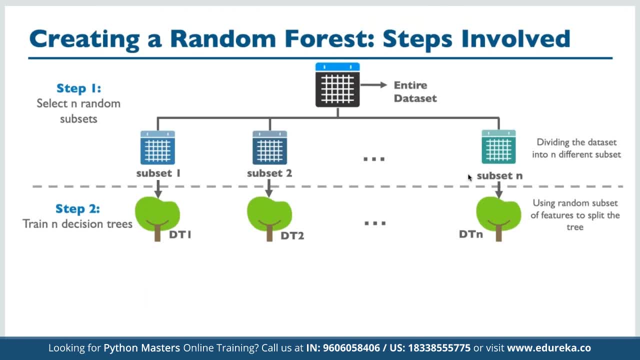 So we then train n number of trees. We provide this each subset to each individual tree. We have randomly selected columns for each split on a tree. once that is done, We know the result of every tree. we then take the voting for every data point, and that's wherever we are getting the 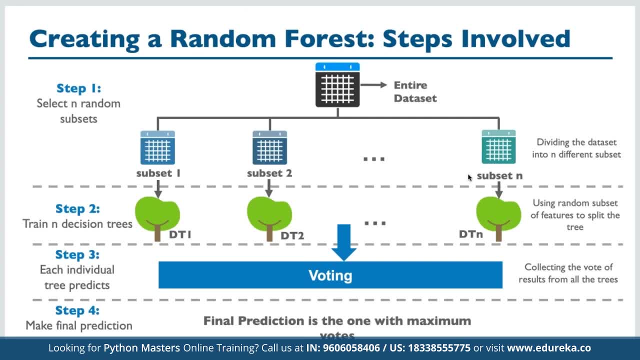 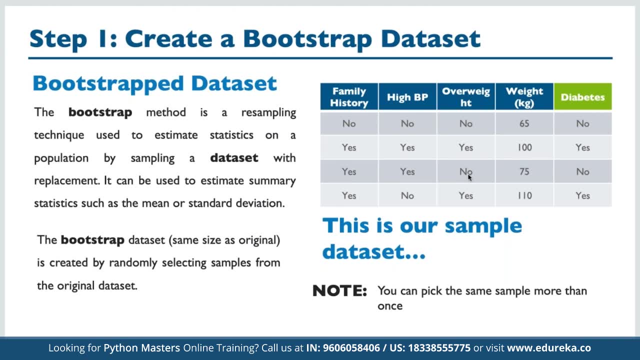 majority of votes. That's the class which we assign. So that's, at a high level, how we create a random forest. This is, you know now, example of creating these subsets of data. This process is called bootstrapping, the creation of subsets of data. 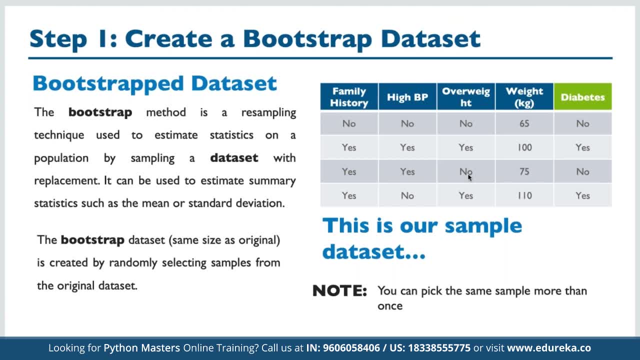 So, for example, the same variables we have now. I have four different rows. So what we'll do is we'll create subsets. every subset will have four rows only, but we'll pick them at random and some of the subsets would have the repetition on different rows. 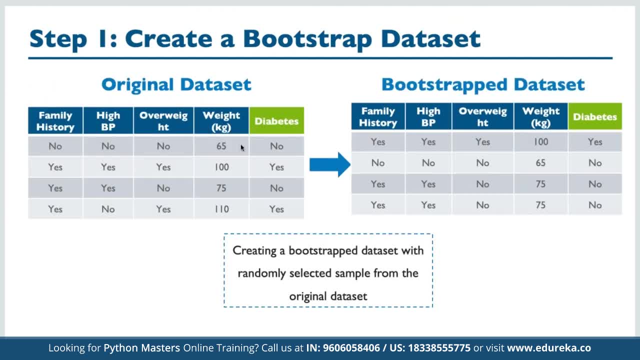 So let's see how it looks. For example, this is one of the data sets. Okay, on the left hand side I have the original data and on the right hand side I have the subset. So, if you see, we have four rows in the subset as well. 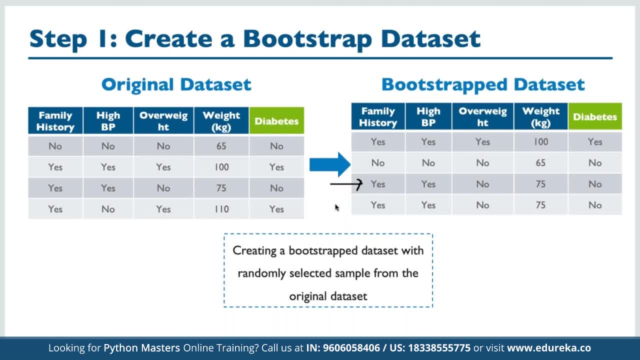 However, this row here and this row here are repeating, So this row 75 has been taken twice, which means now some- some tree- will take these two rows only and repeat them both. some tree might take first and fourth row and repeat the fourth row thrice. 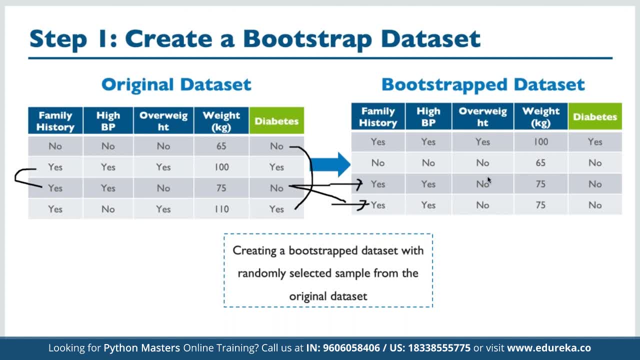 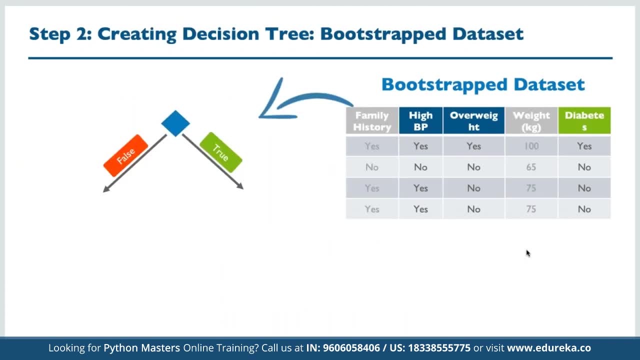 So this kind of permutation and combination will occur and you will have n number of subsets. So this is what is called bootstrapping of your data. Now, once you have your bootstrapped data set, So this is the same data set which this is the same subset. 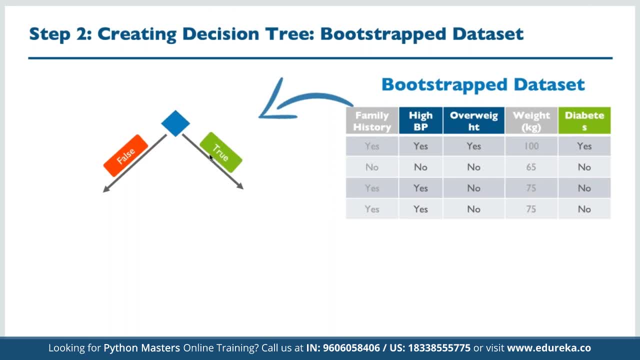 right with two same rows, And this time we are training a decision tree on this data set, but we are not taking all the columns. So here we are only taking these two columns and we hide these two columns from your decision tree, So these two columns are not shown. now this node here will split. 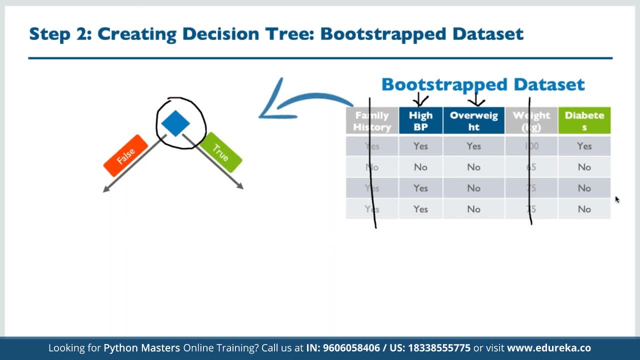 your data based on these two columns only, and the next tree can get a different kind of a different set of columns right, and that process will continue to happen until so. as it says, instead of all the four variables we are going to take only two variables. 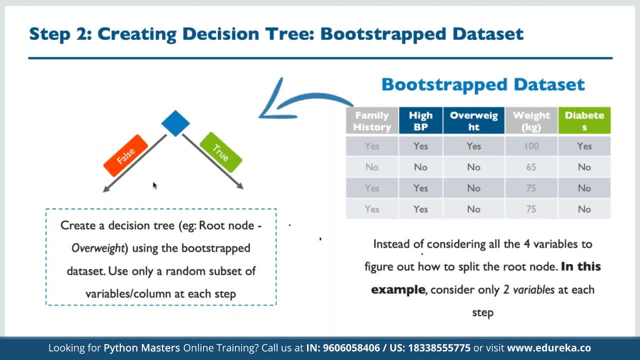 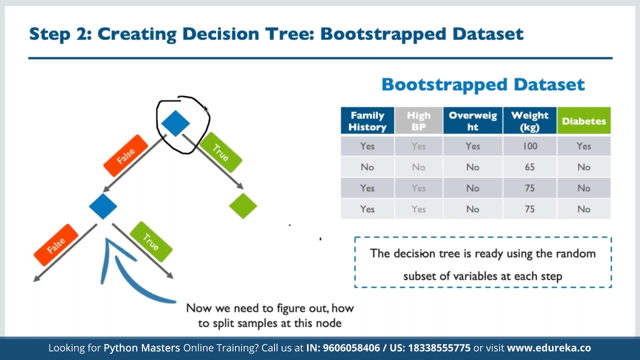 This is your, your bootstrap data set. So we are taking bootstrap data set using random columns, subset of the overall columns, and then building a decision again on the next node We can again take a subset which, and you know, suppose this was partitioned on high BB on the next node will hide this column. 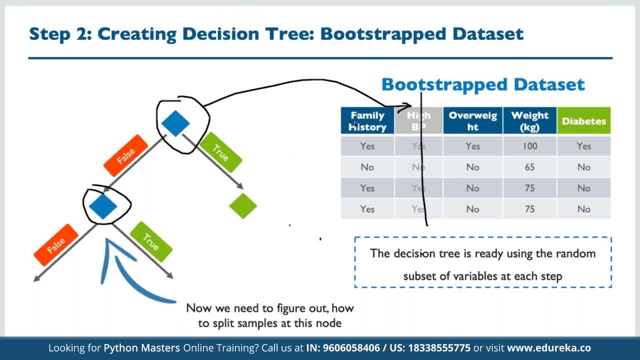 from this. next, you know no will will offer these three columns And, as I mentioned in the beginning, based on different algorithms, like you know, genie index. you can read about these when you study decision trees or entropy or variance reduction, So automatically. 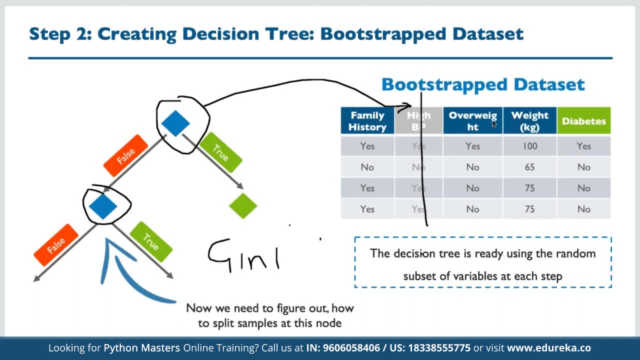 it'll pick. pick which is the best column out of the columns which you are exposing it to will make your data pure, But the idea is that we are letting different nodes take different columns to do the splitting of your data. That's why most of your decision trees will be different from each other. 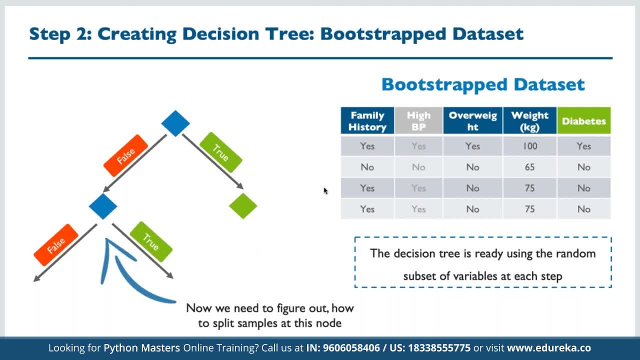 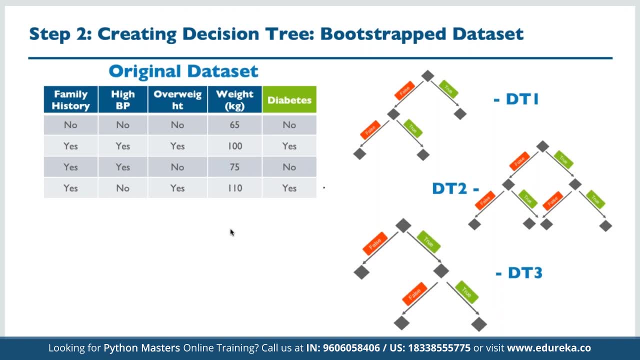 That is the important concept to understand. So eventually, what will happen? your original data Would be used through different data sets to create multiple decision trees, and all the decision trees will be different from each other. You keep on doing this until you have significant number of trees. 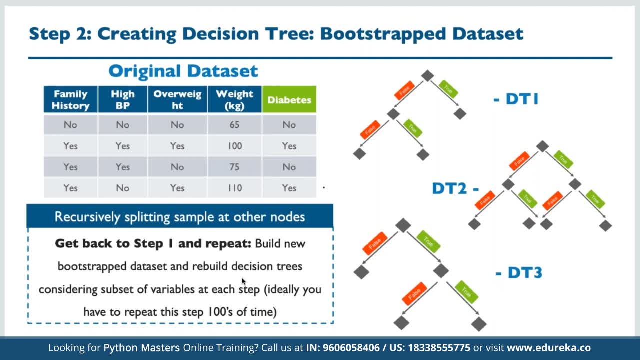 For example, here it says: ideally you should have to repeat this step hundreds of time, because we are talking about a real scenario where you have a lot of columns and lot of rows and, in a real, real practice, real projects. you would. you would see there are. 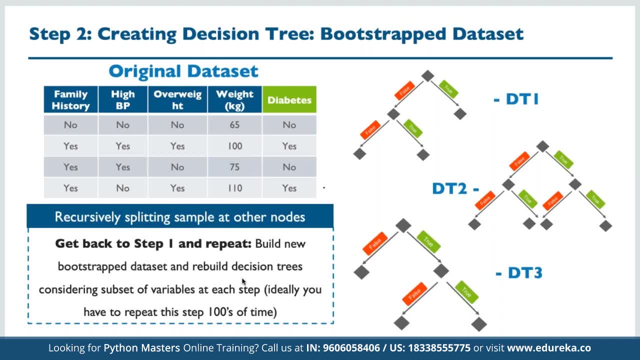 you know more than hundred Variables. there are hundreds, hundreds of thousands of rows there. This kind of algorithm will make a lot of sense. But then you have to create a lot of decision trees. And when I say you, you don't have to do all of this manually, right? 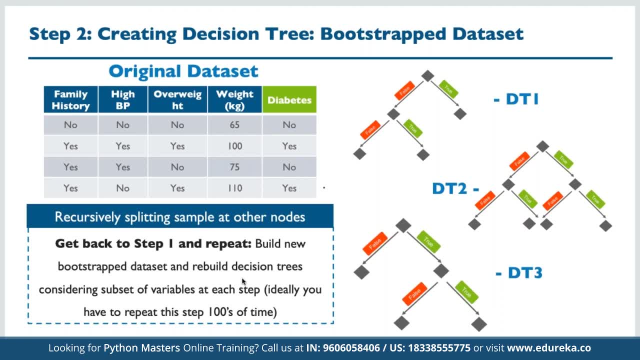 You simply take a function and your function will do all of this for you, But you need to know what is going behind this one, What is happening behind the scene, and then you have to change the hyper parameters, and you can only do that once you understand all of these. 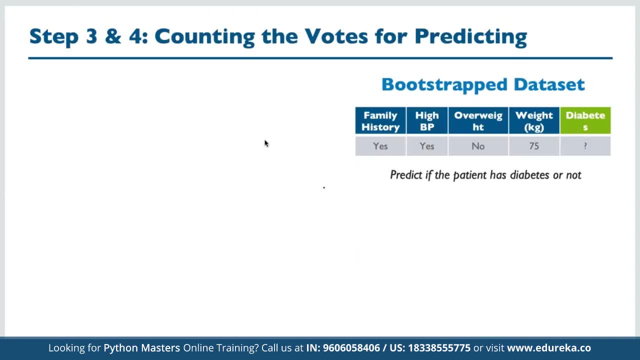 you know details. the last Thing is we are now going to take the votes. So this is data set, which was the same example which we looked at, which was repeating. now, what we'll see do is we'll take this data row and we'll check each and every three, whichever tree received this row. 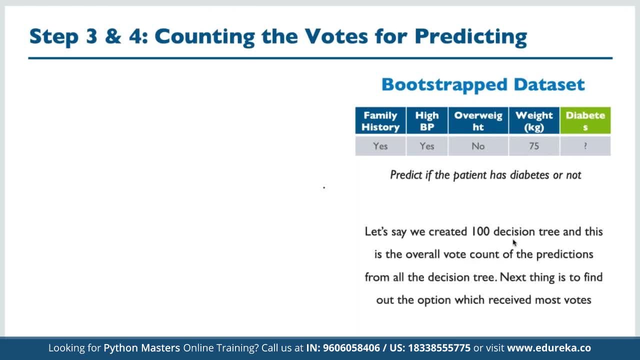 in the data set and we'll see which class that that tree has predicted. So if out of hundred trees, 95 have predicted this as yes and five has predicted this as no, will take this as yes. Now you would ask me what if there are 50- 50, or what if 60- 40?? 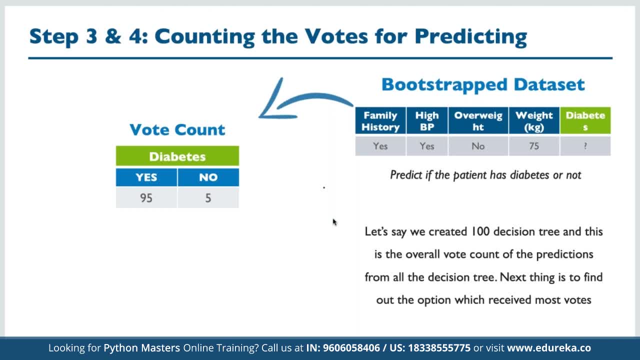 How do we know? you know which to take, but if you think intuitively, this data set is, you know one of the rows from the data set. so that kind of situation will never occur. most of your trees will be predicting it in the right class, only right. 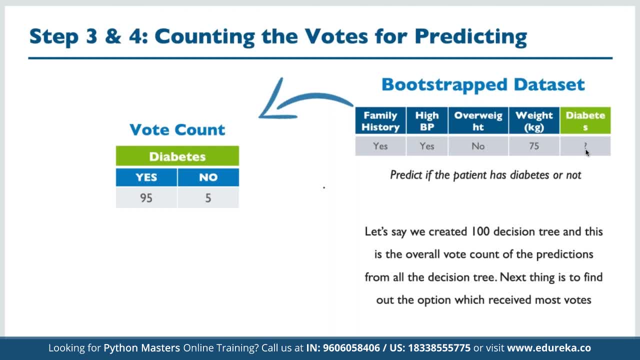 intuitively. if you think about this, there is a significant relationship between these attributes and this class. Only there will be few trees which are, which have you know, used specific set of columns, due to which there is a wrong prediction, but this voting actually is the thing. 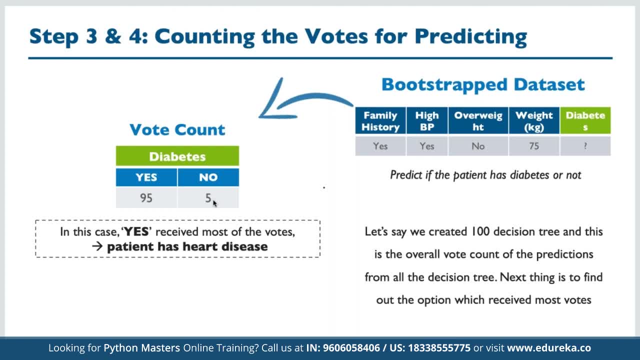 which gives you a very high accuracy when we use random forest right. So you will never get into situation where you'll get 50- 50 boards for most of your data set. If that is the case, what will you do? You will change the number of trees that you're building, even though 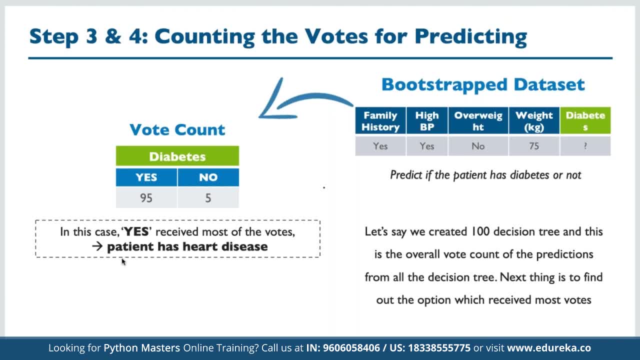 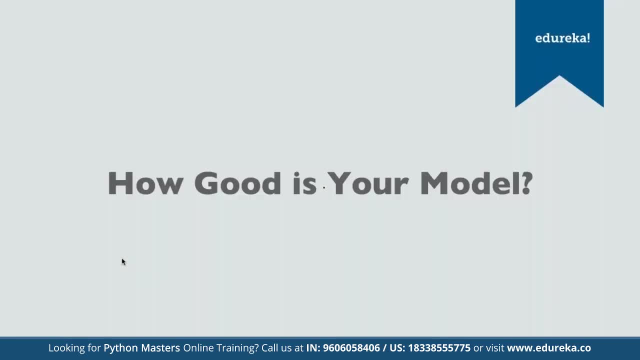 that never happens. But if you continue to face this problem, you know you are not taking the right algorithm. You would switch to some other thing for sure. then the last thing which we need to understand about this is: how do you test that, how good your model is, with the example. 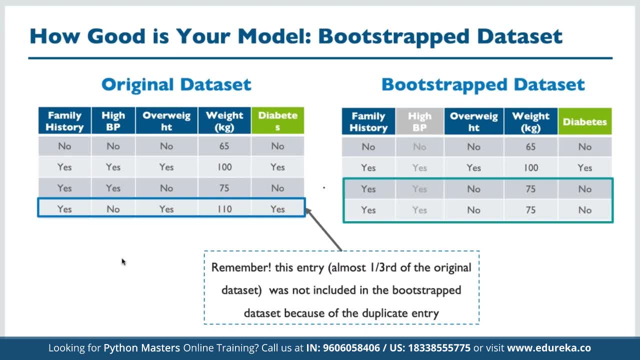 which we looked at. we only created one subset of data in that we did not pick the fourth row. now in in real practice, when you are implementing this, you are going to notice that around 25 to 30% of your data is never picked by any reads. 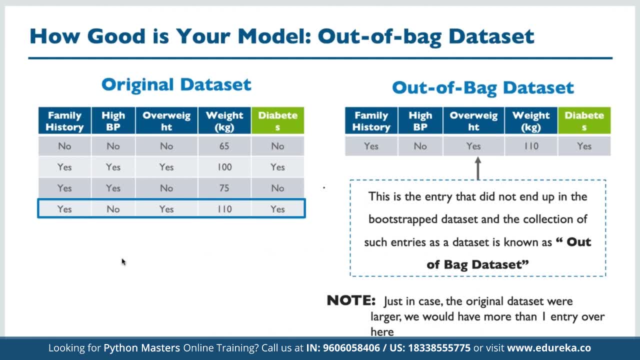 that data is called out of bag data set, which means there are some of the trees which have never seen this row. now, unlike other algorithms where you have to, you know, do multiple iterations of training versus test split, here What you will do is you will use out of bag data set. 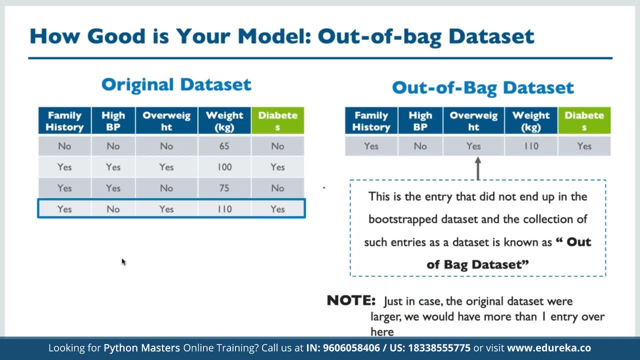 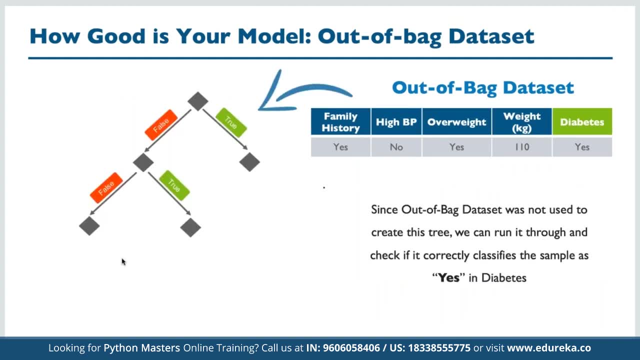 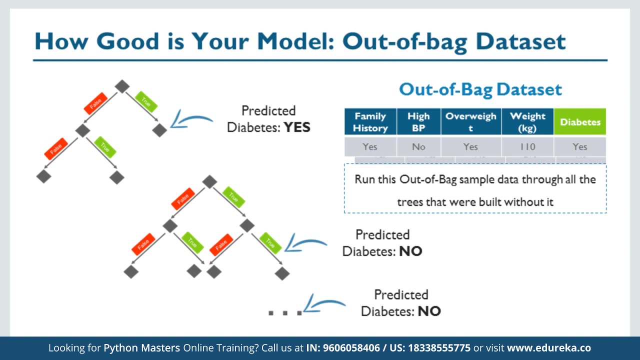 as your validation data and you will pass this to the trees and they will predict this value based on the learning they have done, and again, you are going to use the voting in it, and how many number of trees are predicting this class correctly would become your accuracy. 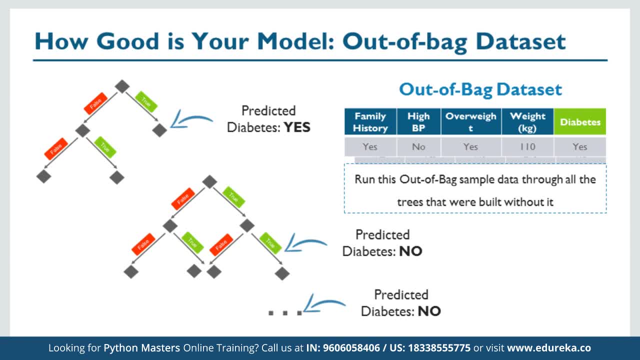 So let me quickly reiterate what I said. There would be some rows which are not exposed or which are not given to the trees because of the random sampling with replacement. in the first example, We saw that that tree received only three rows out of four rows. in practice, 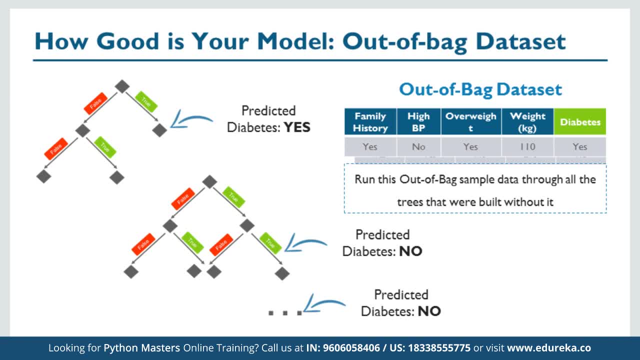 from experience and telling you that there would be around 25 to 30% of your data which will not be picked by the trees. So when we look at one tree and we see that this, these are the 30 rows which were not exposed to this tree. 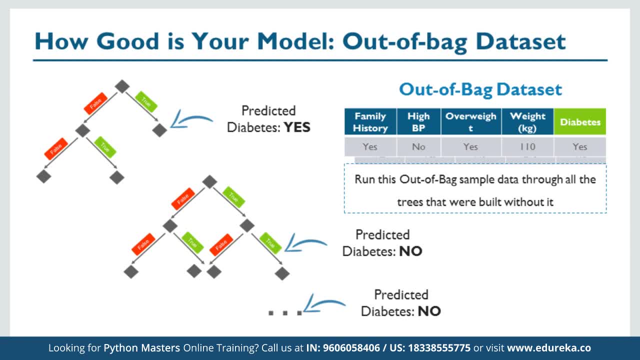 We are going to run through that tree with those rows and we'll see what that tree predicts. We are going to run through all the trees which were not exposed to those rows and we are going to vote. take the vote from these trees and that becomes our prediction. 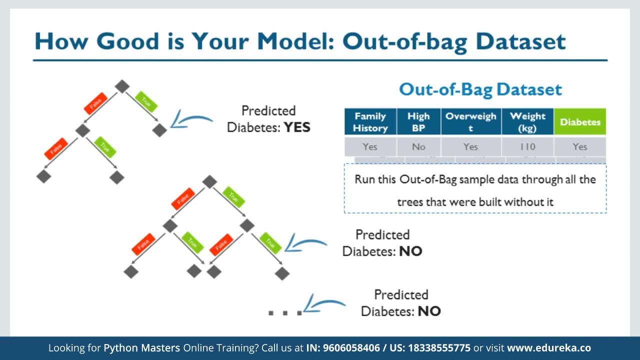 Now we compare these prediction with our actual values and whatever right predictions have been made. that becomes our accuracy of the model. And of course here also you'll take care of your precision, recall, F score and other matrices. But for simplicity I'm just taking example of your accuracy. 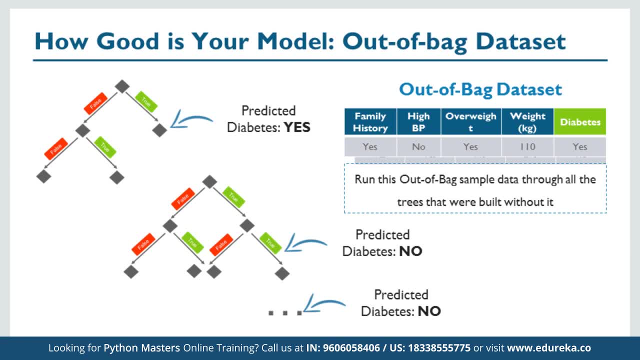 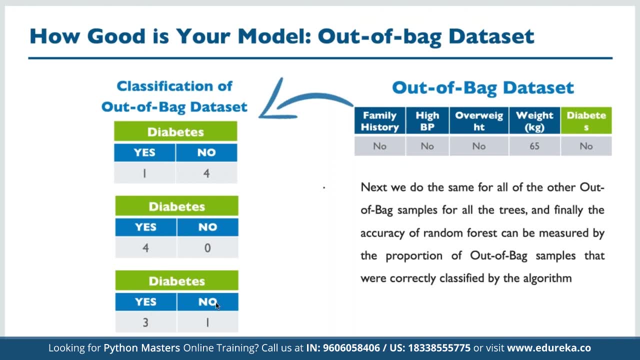 These are called out of bag data set, So it may happen that you know you ran it through a set of trees and then in all you are getting like eight yeses and five nodes for your this specific row, and you know this row has been predicted wrongly. 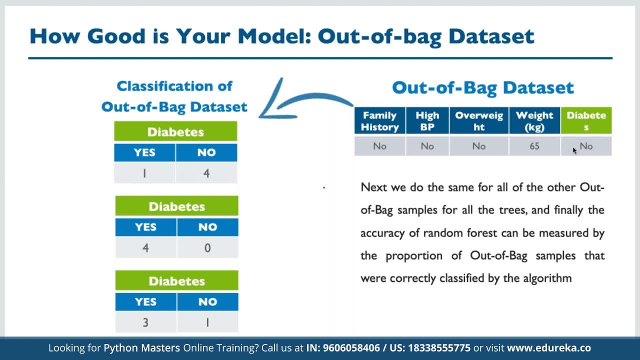 because you are getting higher Vote on yes. So eventually you will. you will, you know, take this as your false positive- or false negative, depending on whichever class they belong to- and this will become the reason for lowered accuracy. So all these kind of cases will be part of your denominator. 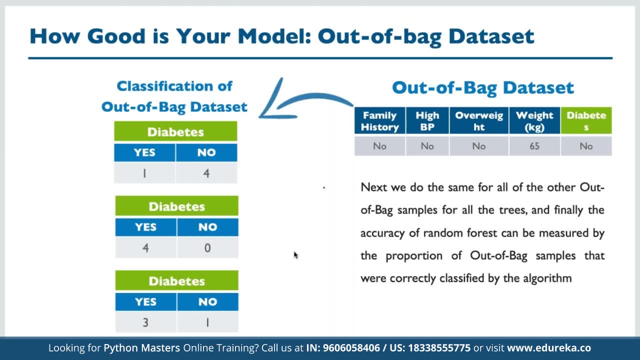 not the numerator when you calculate your accuracy, but this is how we check your model accuracy and, depending on your initial confidence level, Etc. If this accuracy is beyond that threshold, like maybe 90%, 95%, 99%, whatever is your threshold, 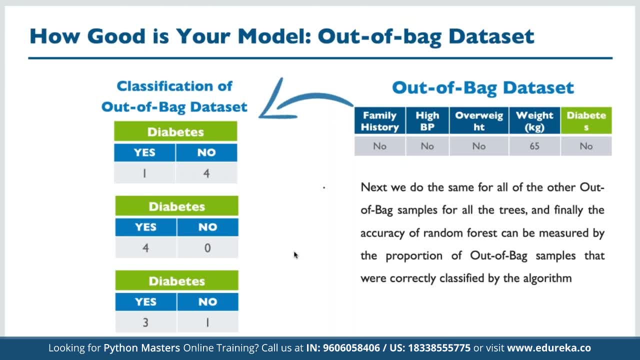 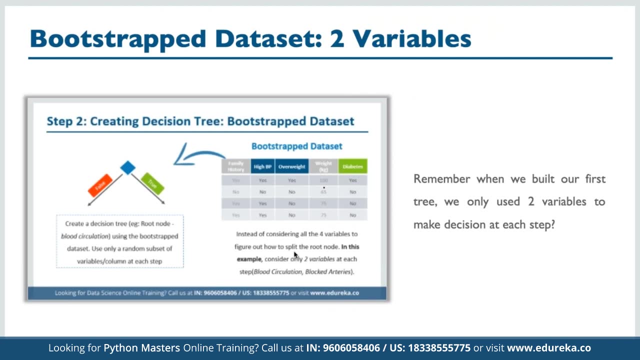 then you would say that your model is working fine. Otherwise you have to retrain or or, you know, do the tuning, Etc or pick some different models. Now, if you remember, in the first example we looked at two variables to split your node. 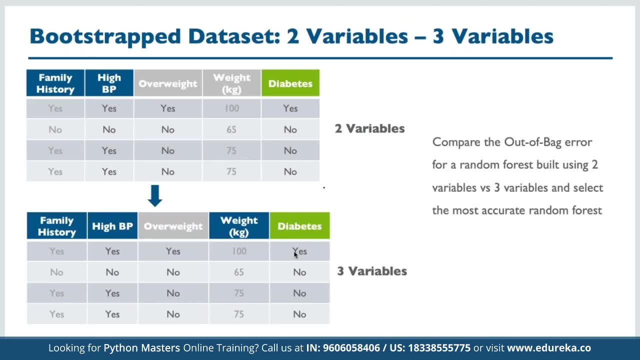 You can pick between different number of variables. and when you check your accuracy then of course what you do is in different iterations You do different variables. So first you'll build, you know, trees with two variable. you build with very trees with three variables. 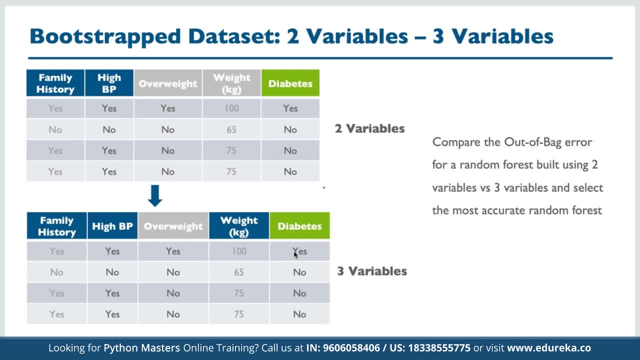 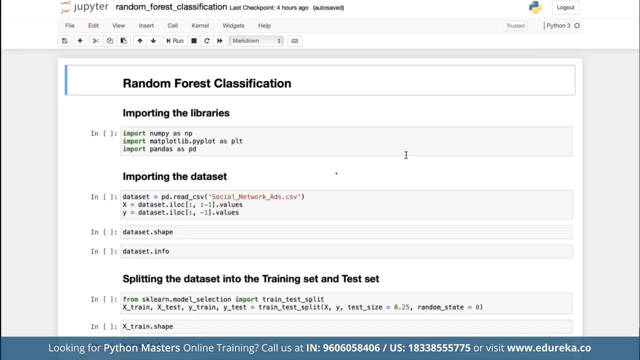 whichever set of trees is giving you better accuracy. That's the number of variables You are going to pick for your training of your trees in the next iteration. Let's now move to one quick demo. So in in python, Or, or, are, or says, for example, to achieve one task. 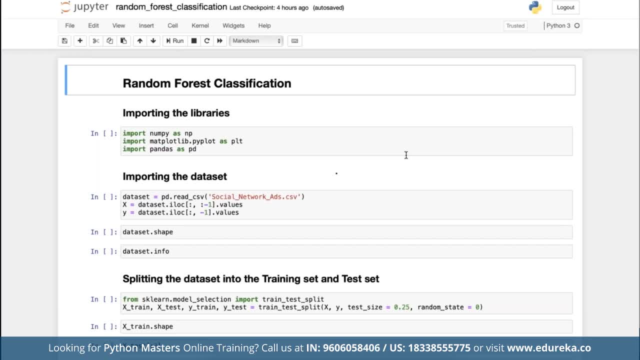 There are always different in multiple ways. Okay, you can. you can do the same thing with multiple functions. All of them will give you the same results because these are open source and you know there are people who keep on adding different libraries and functionalities. 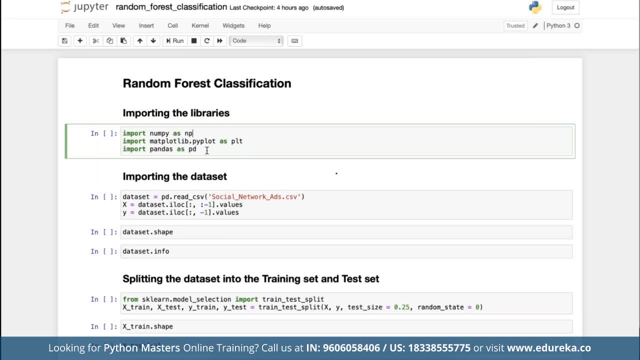 So let's do this. I'm importing first the three basic libraries so that I can work on the data set numpy for all the algebraic applications on matrices. pandas, for you know, deal with the data sets, like tables, are converted into array based data frames and format matplotlib for any plotting. 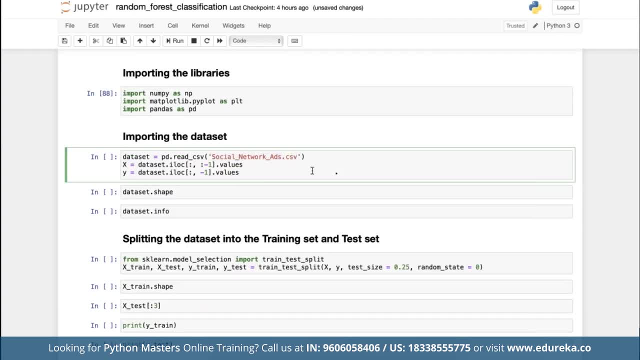 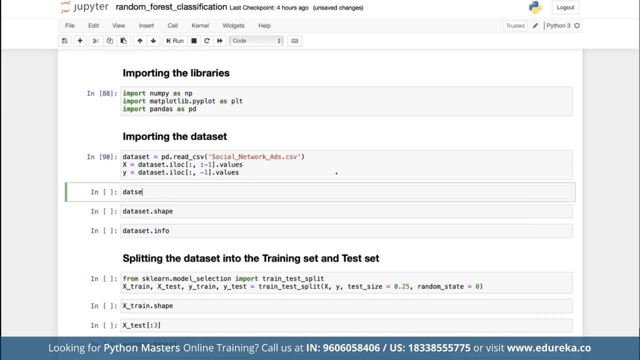 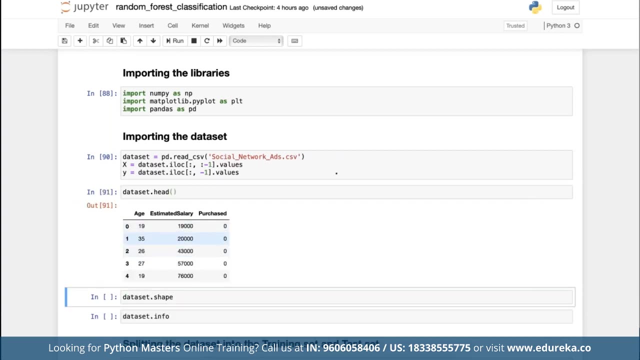 So we have a small data set which is again for classification. So I'll quickly show you what. what do we have in the data? So Right, so we have a very basic data set. We have just two columns, which are independent: age and estimated salary. 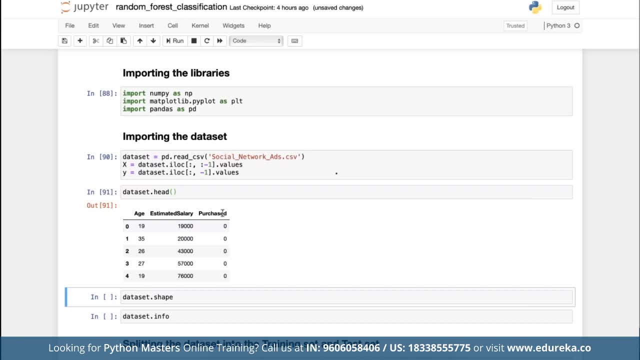 and based on these two, we want to predict whether somebody will purchase something or not. So here we have already a label available. So this purchased is the class which can be 0 or 1. 0 might be representing that they will not buy and one will, you know, show you that they will buy. 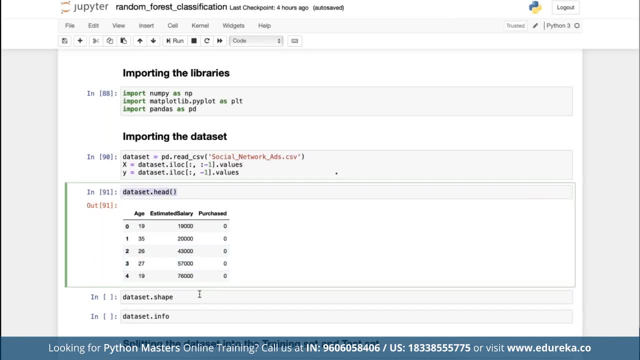 I'm simply showing you only the first five rows of the data. Okay, if I look at the shape, for example, we have 400 rows out of it. Some would be 0, some would be 1.. So this is the label data. 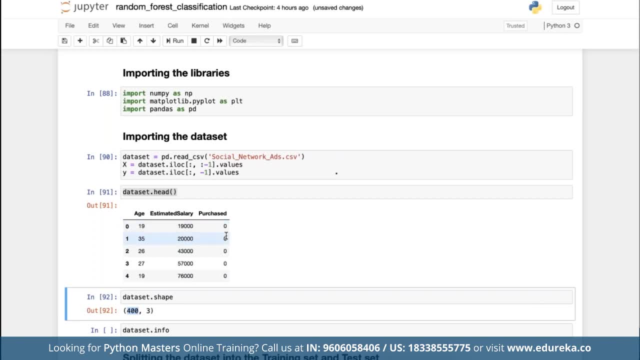 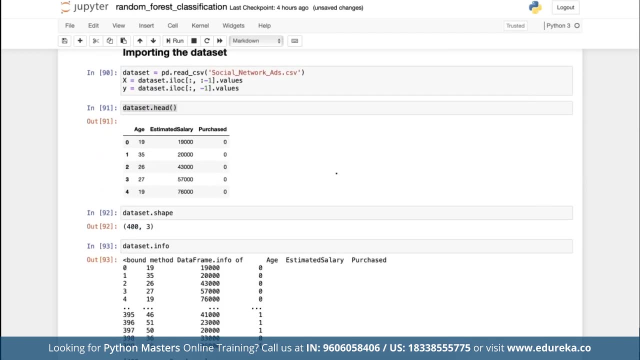 because it's a supervised learning algorithm. I need to have labels so that I can train this model on this data. I basically have, so let's see the info also. So here we have for some of my rows here. It has the label as one type. 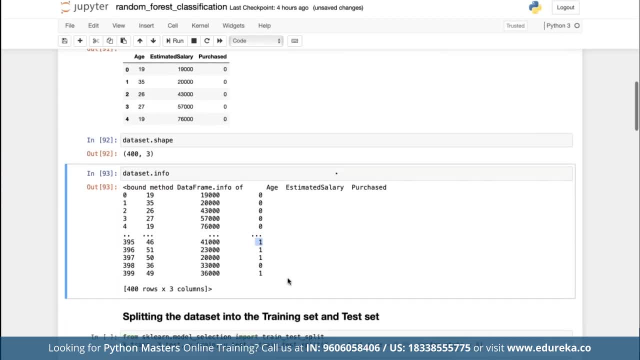 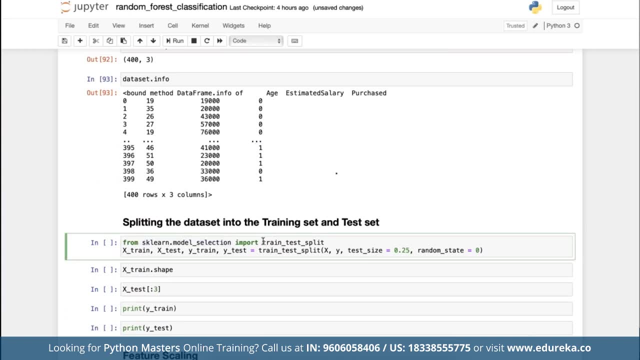 which is the purchased class, So I have just two classes, even for now. what I do is in scikit-learn. I have a very nice function which is used for splitting my data set into training data and validation data. even though we can, we can validate on out of bag data set. 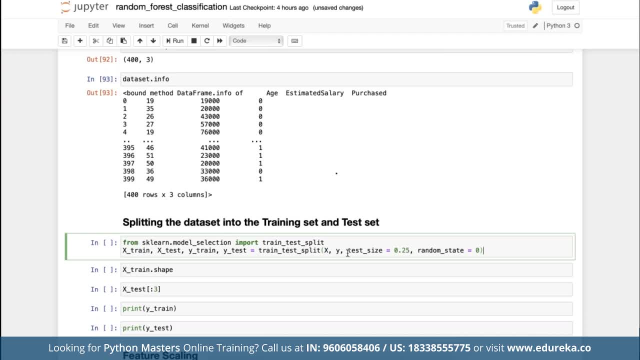 which it automatically will do for finding the accuracy, but we manually also should test and we should not expose all the data to the model, for which we are keeping 25% aside. So what it will do is it will create the data sets, training data set. 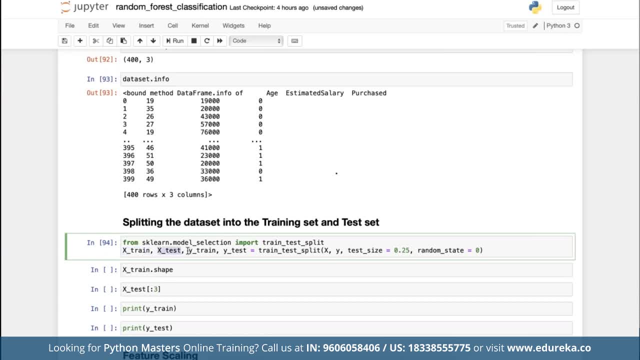 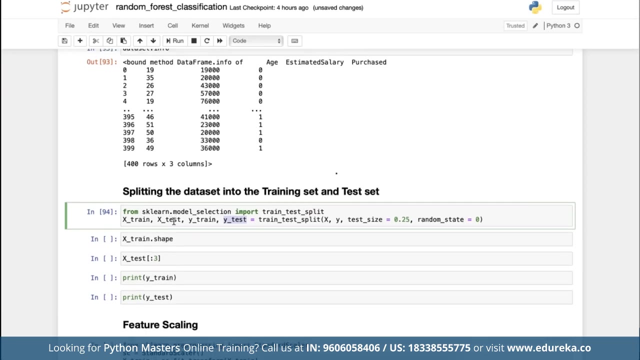 for independent variables, training test data set for independent variable, then by train is for the purchased column which is your dependent variable, and this is will be used with extreme, and then test will be your hidden class values for each row in the test data which will use for testing your accuracy. 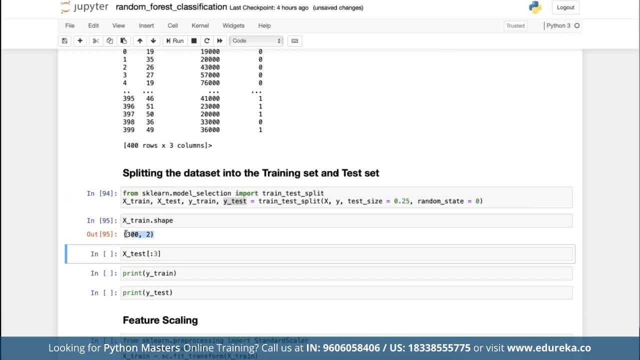 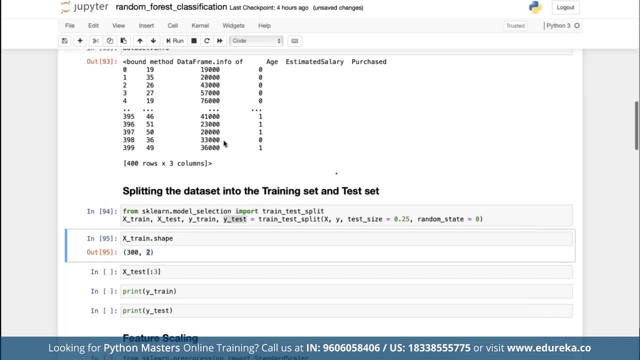 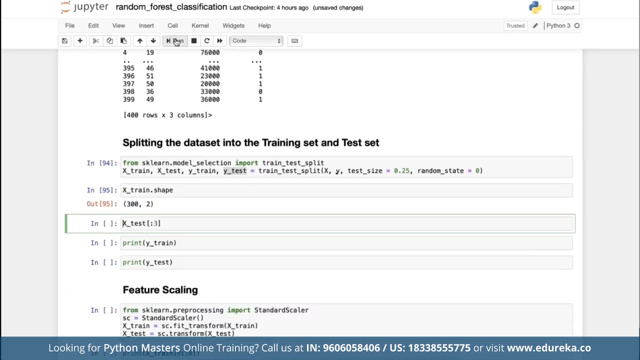 right And now I see the shape. It has taken 75% of the data from the rows out of 400.. Now I have 300 rooms And, of course, we already deleted or removed the column purchase, So I have 300 by 2. if I need to look at the example of sample data, 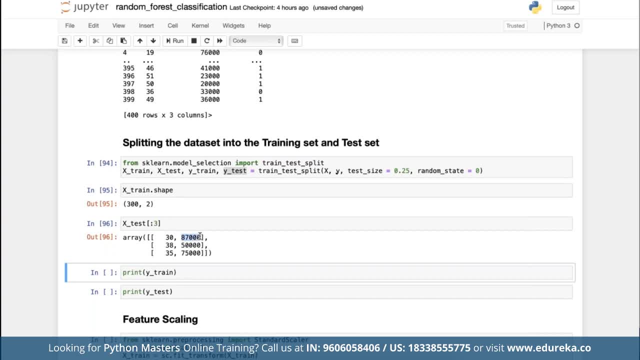 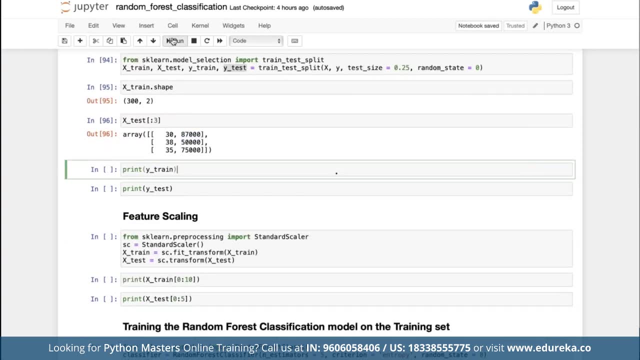 So this is what you we are getting for age 30.. This is your salary. So this is your just three rows Yes showing in the X text and your training. Sorry, why will have just your predicted one ones and zeros? So this is the training data set. 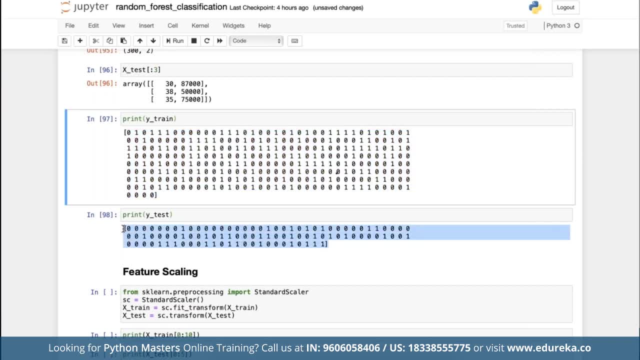 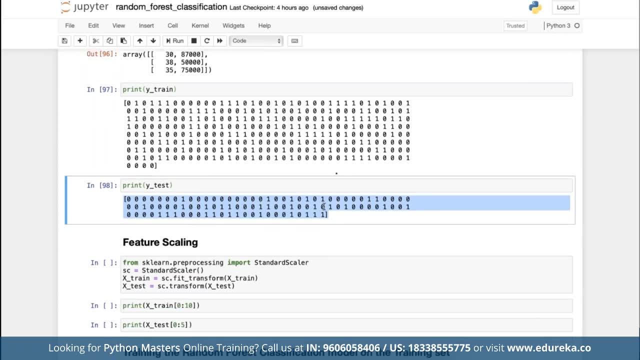 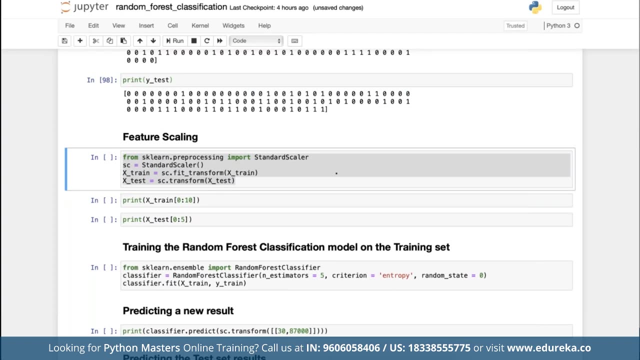 So we are going to give this to the model. This will keep with us and for those rows will then see what your model predicts and then we'll compare against these. That's what will tell us the accuracy, even though your decision trees or random Forest need not, don't need a data to be scaled. 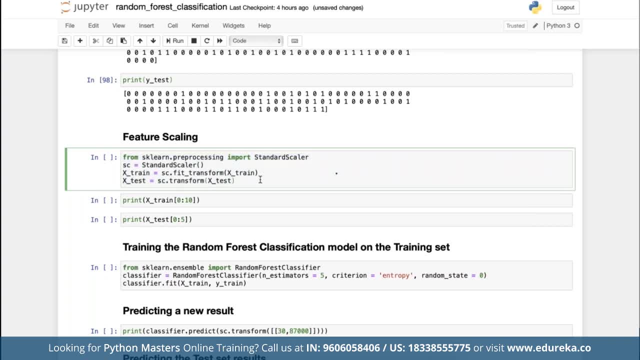 But here we are scaling it for the purpose of visualization so that we can, And you know, accommodate them on X's. So we are scaling this data. by scaling We mean we are trying to bring, remove the unit from your data and bring them close to you know. 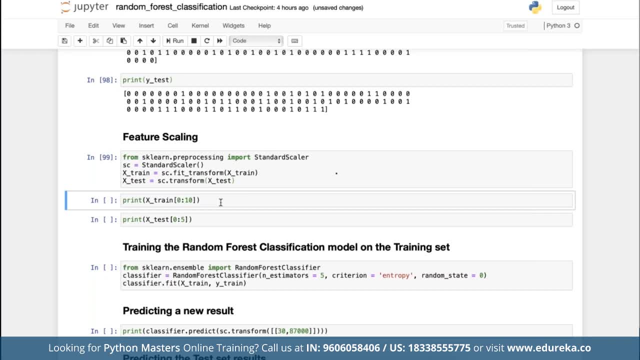 small values between. generally, we are using standard scaling, which will use the standard deviation method, or z-score, if you know, in statistics. So your values will primarily be between minus 3 and plus 3 and, irrespective of the size of the data in units, They all will become similar in nature. 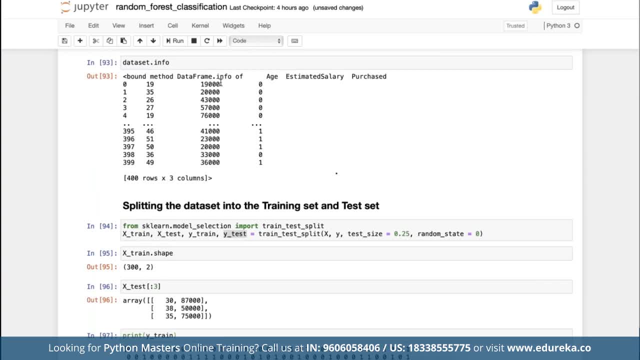 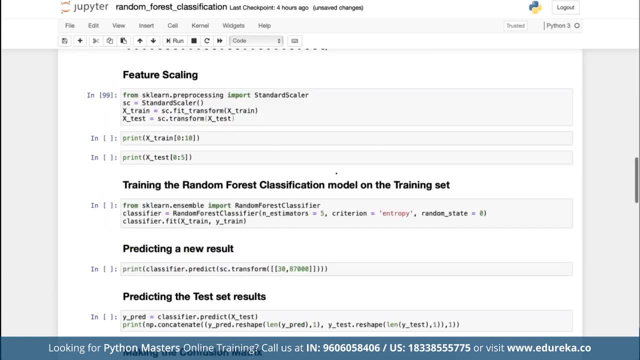 For example, in the real data here, age is a two-digit number, Salary is a five-digit number. But when we scale them, all of both of them will become a very small number, right? so we can easily visualize them. So there will not be a bias in the images. 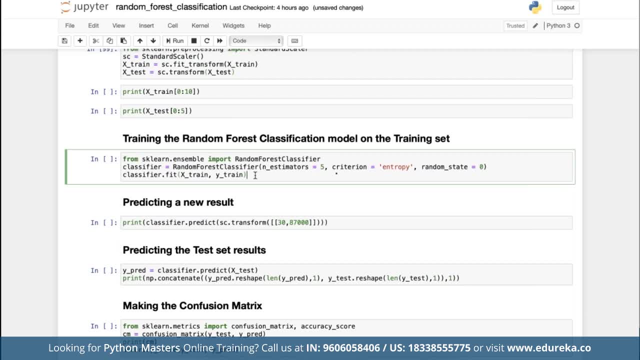 Now there are some models which need the data to be scaled before they can be implemented, unlike decision trees. So here we don't need to, but here we are doing it for visualization perspective. Now, as I told you, we can use different mechanisms for splitting here. 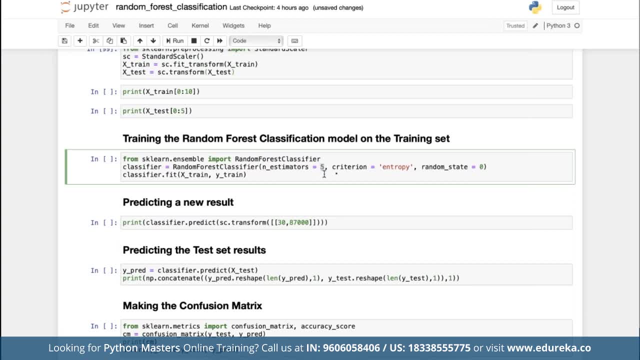 We are using entropy and we are simply creating only five trees because we have a small data set right. We don't have to create hundreds of things. So if you change this, an estimator, you would know how changing your trees is changing your accuracy. 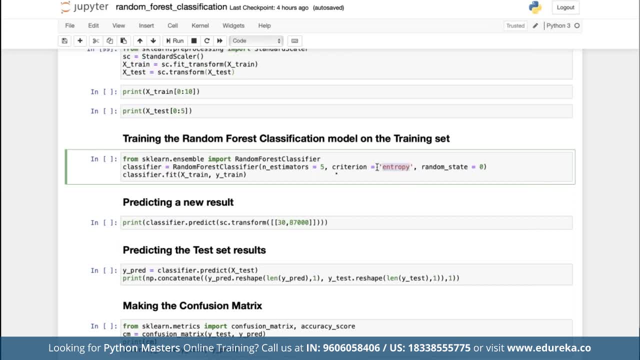 If you change entropy to genie or some other variable which will be implementing the mathematics for splitting, it will also help you in terms of testing, which gives you better results. Random state is equal to zero, So within one programming language. also, as I said, 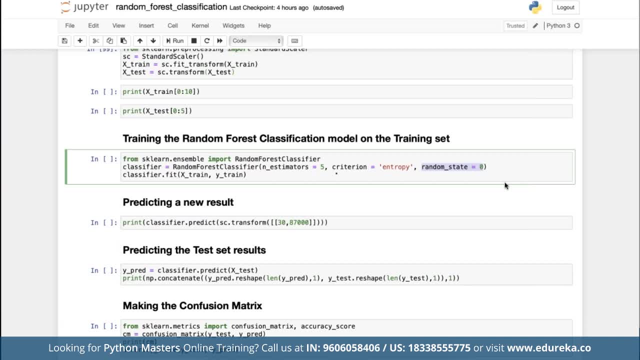 you might get different samples If you don't use this random state. in our also, you have something called set C, which means it always will take the same sample, no matter how many times you run this algorithm. Okay, it will not make impact on your accuracy. 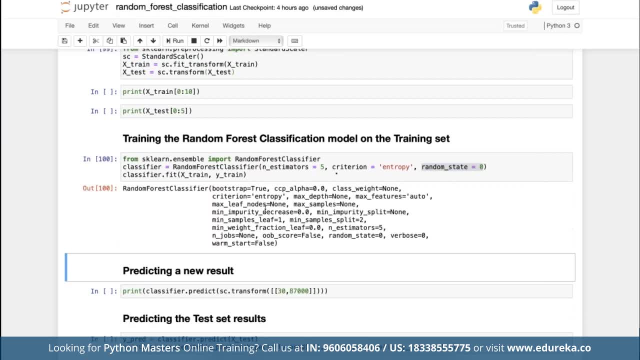 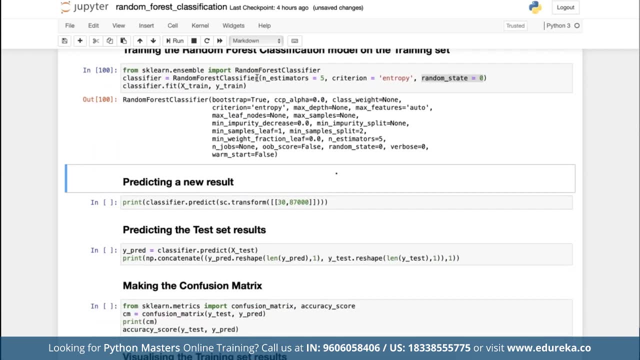 etc. because, as I explained earlier, that will be taken care of due to the Large number of trees which are being generated. So this is: you know, we have Randy random forest classifier on your data set and we have now training that the model using X train and Y train. now, 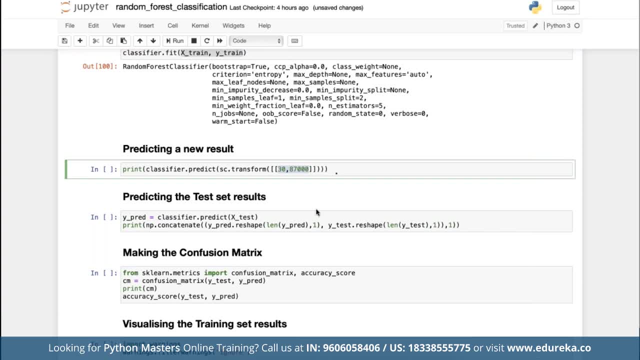 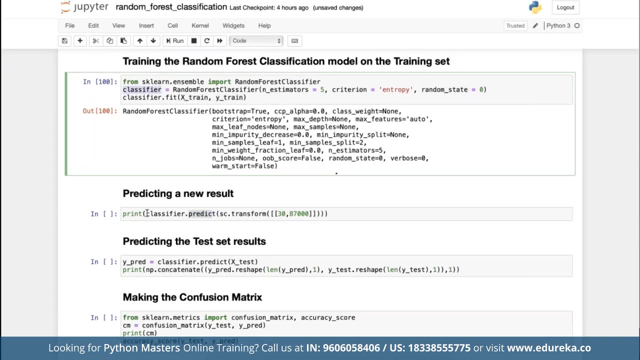 as the model is trained. So what we do is we pick any random data from your data set and then we scale it and then we try to predict using this same model which you have trained, because we have put your model into a variable called classifier. 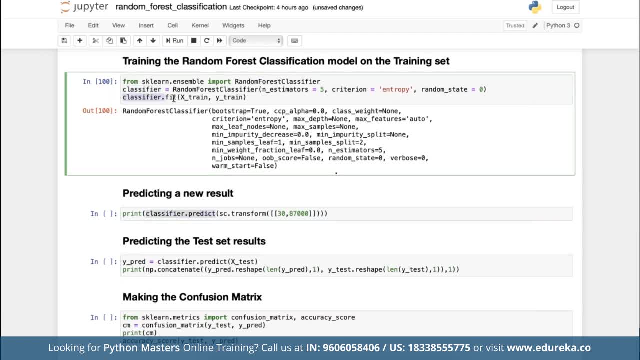 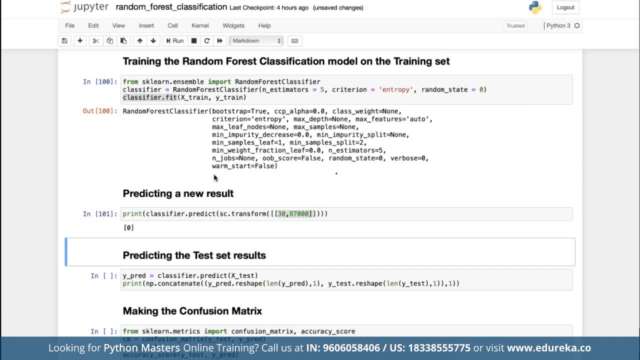 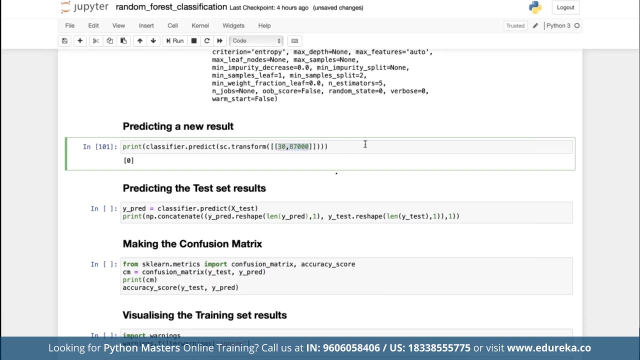 So here we are saying classifier dot predict. here We were doing classifier dot fit. So we are giving just one example. It should predict 0 or 1, depending on whatever this random forest has predicted for this tree. So this is just to show you that if I pass any X value, 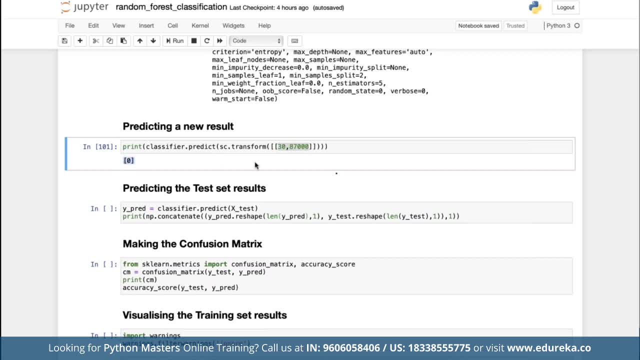 it will automatically give me a Y. So now what we can do is we can go to our data set, We can see what is the actual class for this data and then it will see if it is 0. We know it is rightly predicted if it is one. 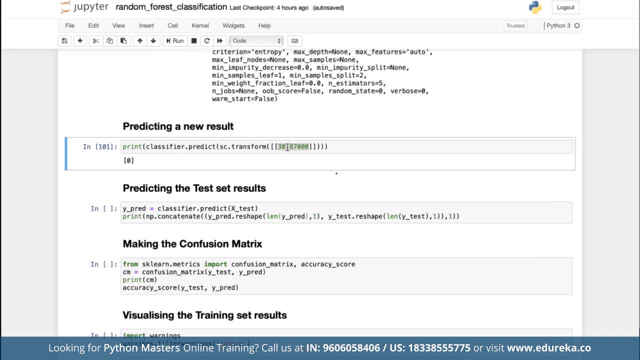 we know it is. if it is different, it is wrongly predicted. but we don't have to do this for each and every data row. So what we do is we take your now we take the test data and we try to predict your model on all of the rows together. 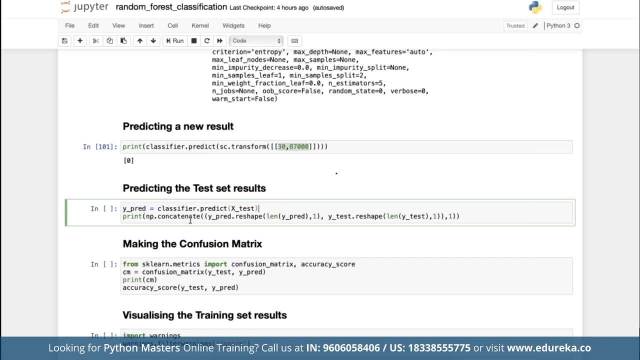 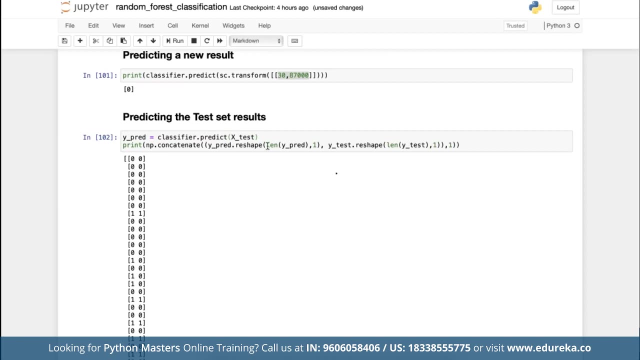 and we are putting that in a variable called by prediction, and then what we'll do is we'll compare all of your actual values with your predicted values in one go. Okay, for which? so this is what we have done. So here, if you see most of so, here we have a first: we have predicted value. 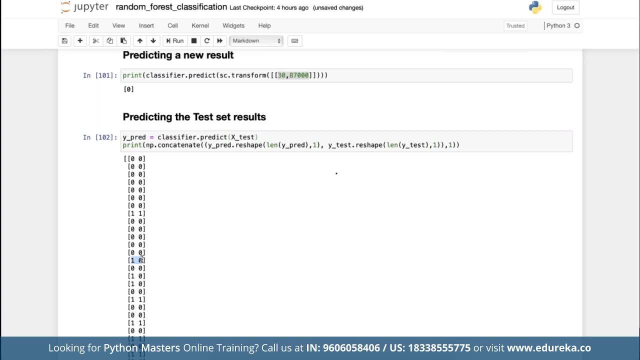 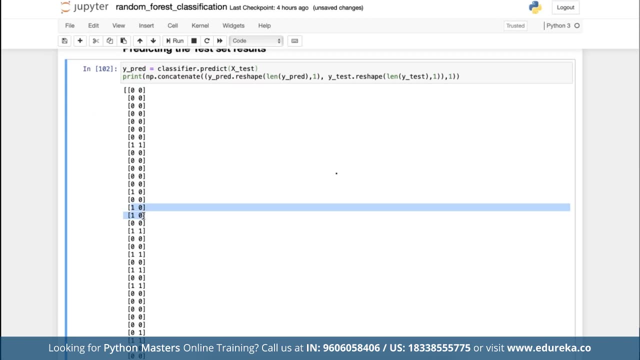 and second is the actual value which we got. So if you look at this one, this is wrongly predicted. so far, I can't see any wrong prediction before this and then we have more wrong predictions here time. So this way you can actually see if you want to look at each individual value. 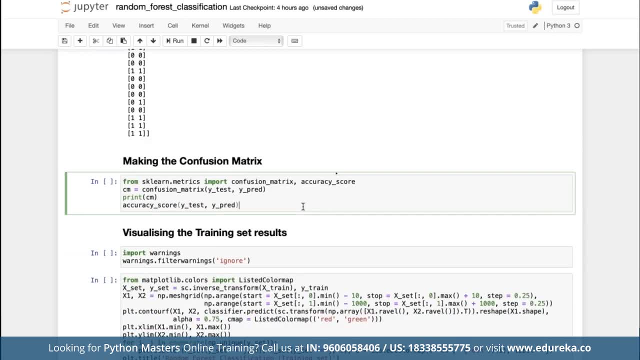 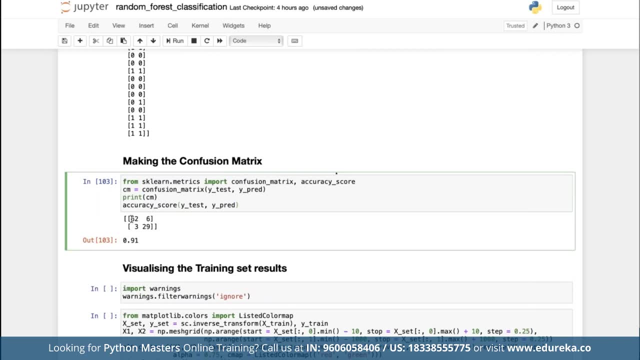 So which one are rightly predicted, What is wrongly predicted? But if you want to, you know, do this in terms of accuracy, Etc. So you can create a confusion Matrix. So now you get a 62 plus 29 are rightly predicted. So, if you remember, out of 400 rows, 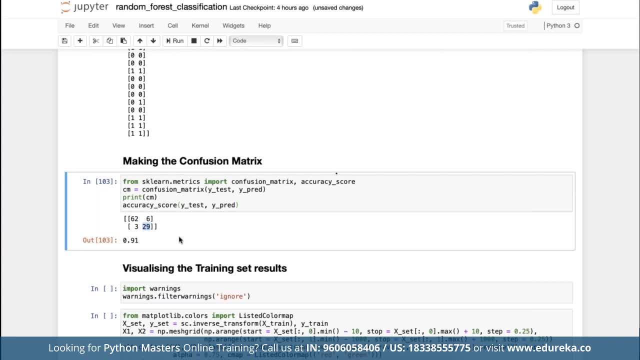 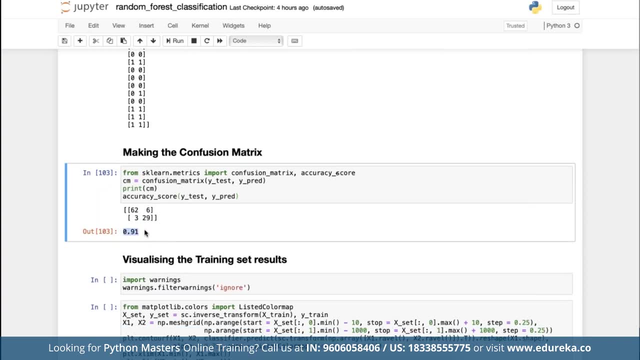 we had taken out 25% for testing, which are hundred rows, So here we are getting 91% as your accuracy. So we can say that overall out of hundred, 91 are predicted correctly, because you see, three and six are the wrong predictions here based on your confusion Matrix. 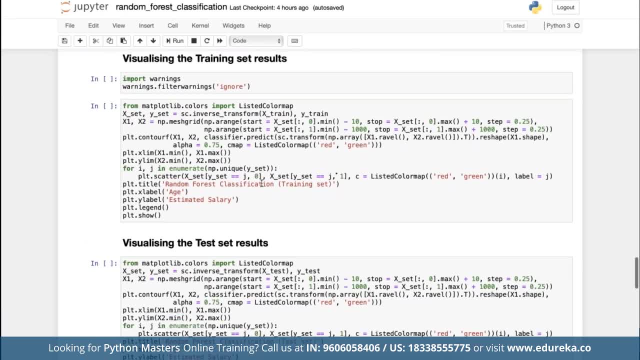 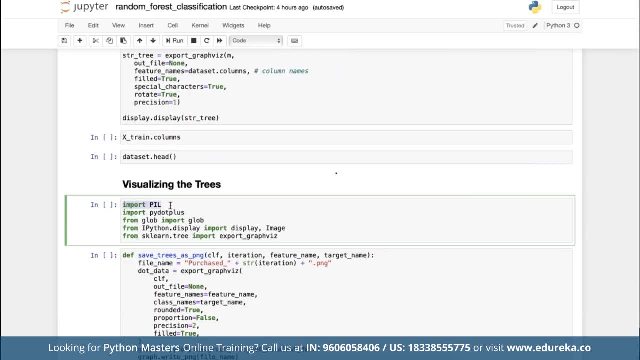 Now, what we'll do is we? let me not visualize this. Let me rather show you actual trees so that it gives you more sense. So import pill, It's a pillow library which is for managing your images by dot plus is again creating files. 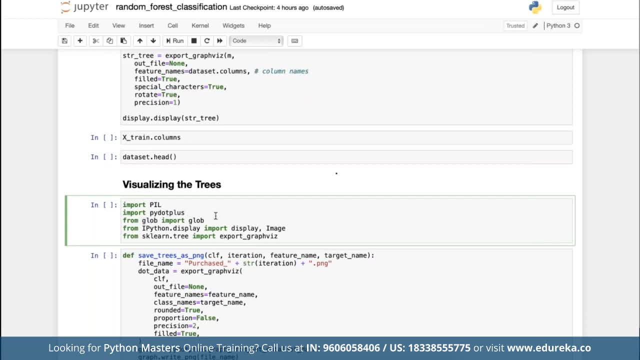 at sector of image images. a glob will be used for a converting a tree into, like the numbers into a visualized tree, and export graph piece is: is you know part of your psychic learn the tree sub module which is used for a displaying any tree or any other image. 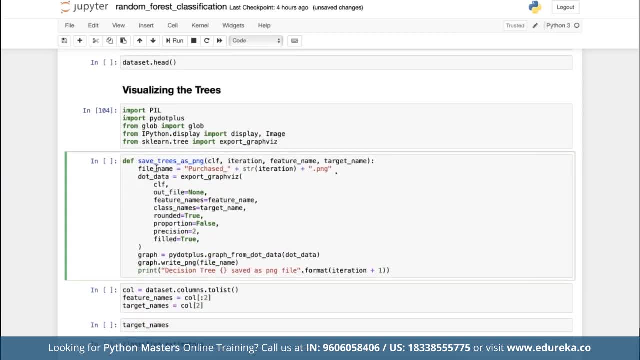 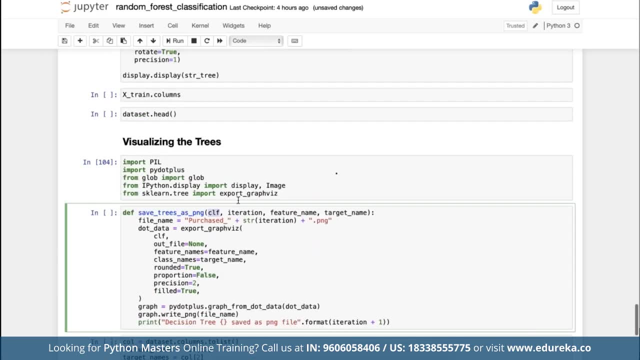 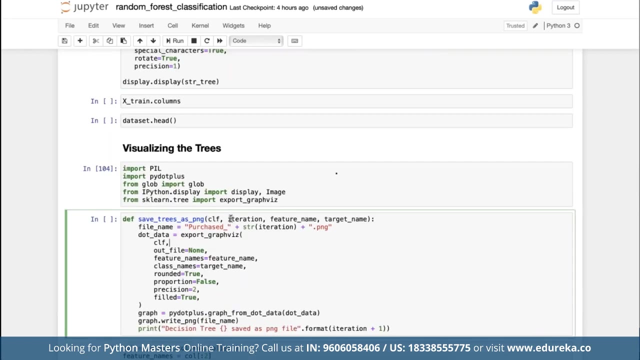 Okay, so I'll import these libraries. now I I'm creating a function called save tree as PNG. It will accept outcome of a model which you know we have seen here, for example. So this will be The first argument to this function. then we have iteration. 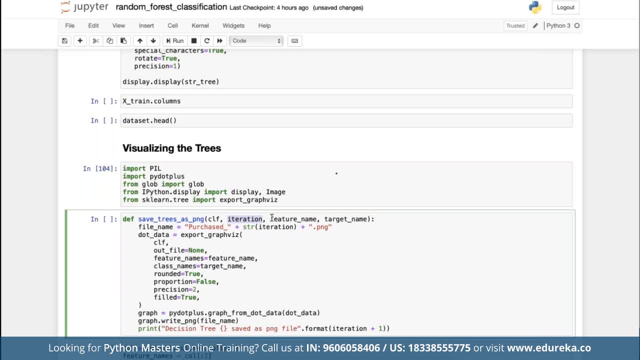 for example, how many trees we want to generate. feature name is the name of your independent variables. here It will be age and salary, and then target, which is your purchase. So what I'll do is I'll pass these four values and then I'll create a file with appending purchase. 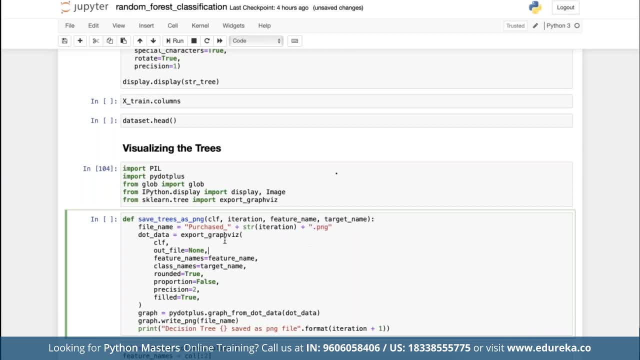 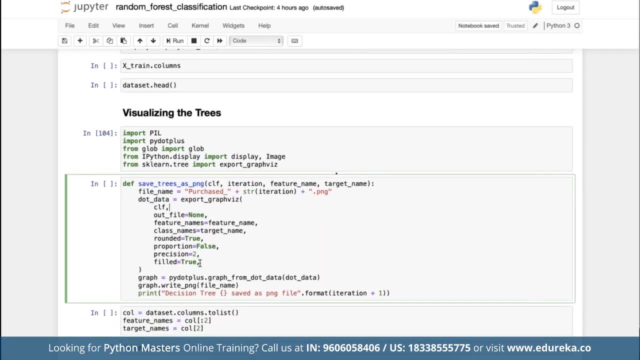 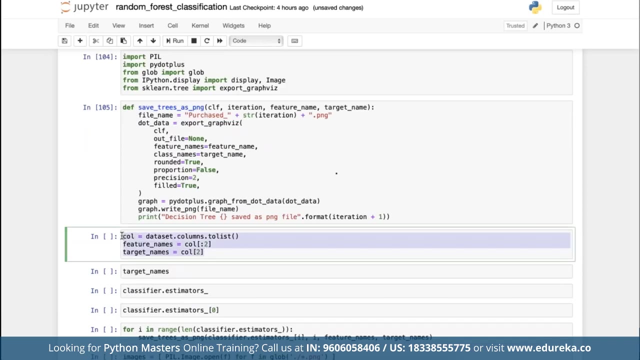 and the iteration numbers, and then we'll add PNG to it And dot data. as I said, this will be used to generate the tree and if I run this now, it will simply create this function, and I am now extracting the feature name as the first two columns of your data set. 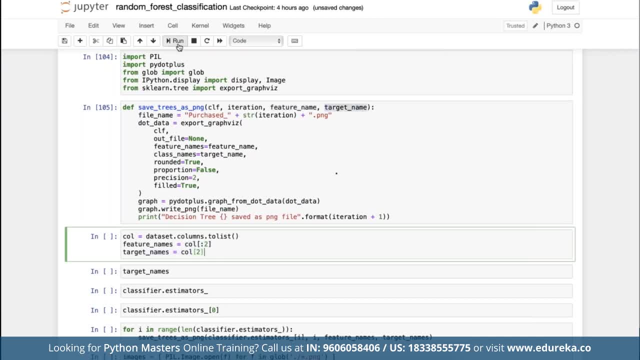 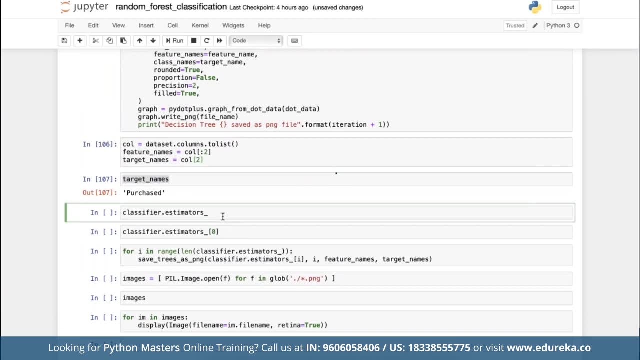 and target name as the last column of the data set. So it will give me these two variables. If I quickly test, target names has purchased. So we are good. and when you ran your, when you train your model, you put that into the classifier variant. 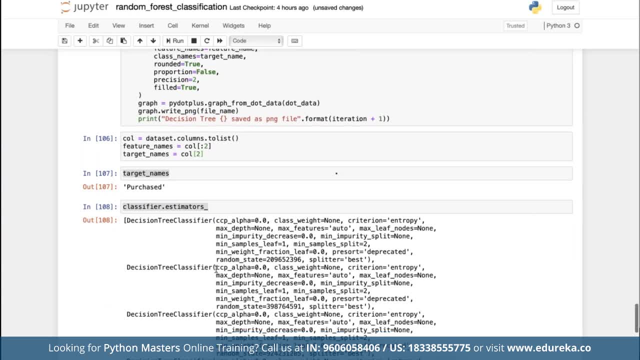 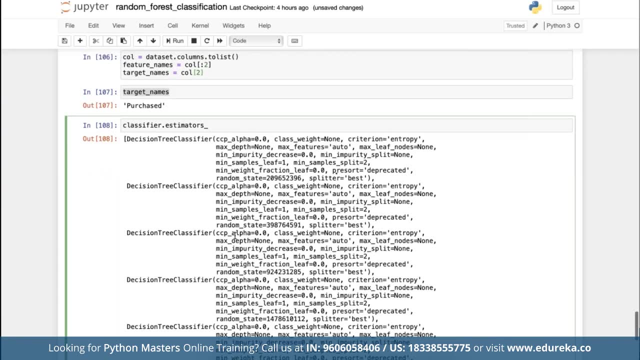 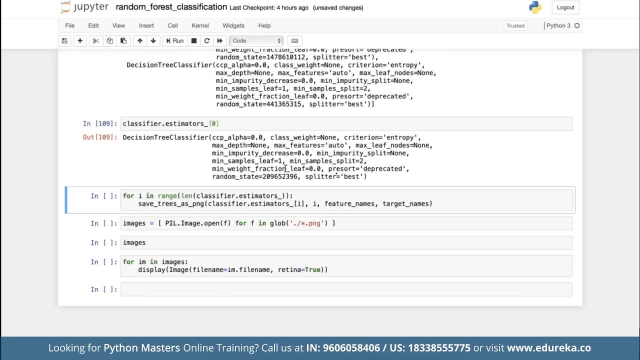 If you want to look at your, you know out output so you can use that with object of this class. estimators underscore. So as we trained, as we created five trees, it is giving us five different tree data. If you want to look at a specific tree, the first one. 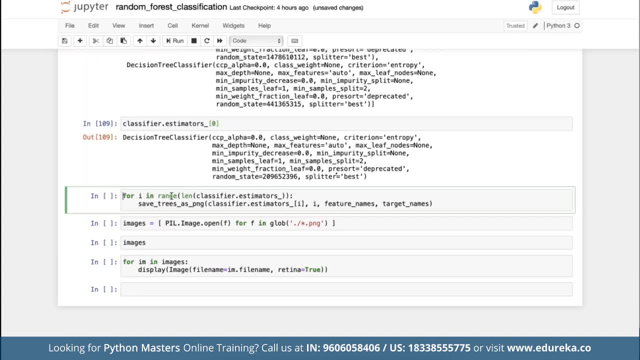 this is the first tree. So what now I do is I run a loop on this length of Classifier estimators, because if I change five to six, I don't want to change this code all the every time, and I pass these four available and I call this function that I seen just created ever. 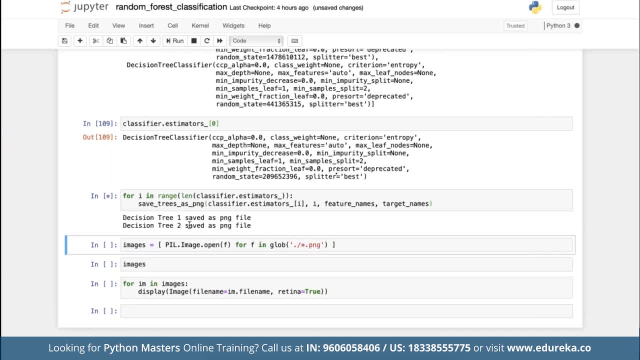 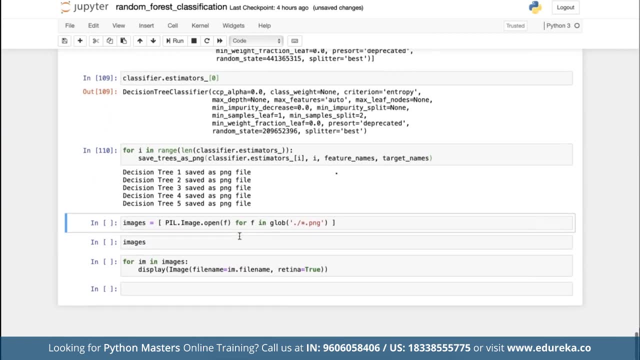 So if I run this, it will create five images for each individual tree and those are created as PNG files. Now, using my pillow library, I'll be able to generate these and I put that in variable Images. So if I show you these are the files and to display them, 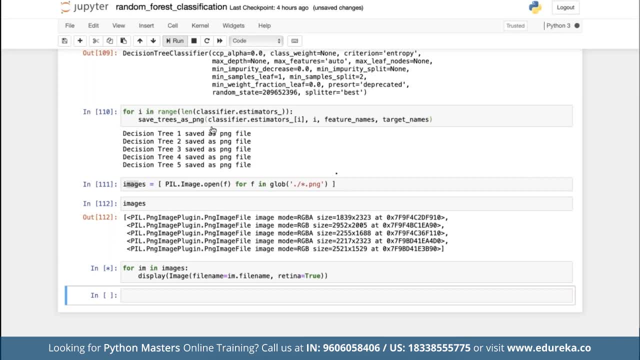 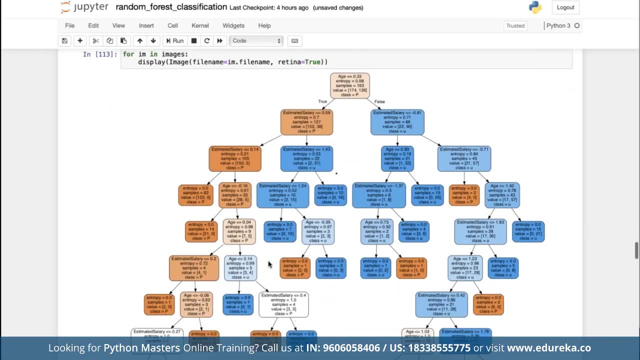 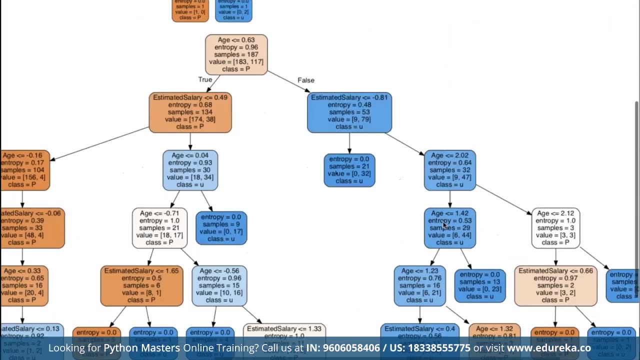 I'm going to use my image function and with loops, I will run this. So now, if you see, this is the first tree, which was which has been built, and then I have my second tree, starting here. If you see, the shape and length, Etc of every tree will be different. 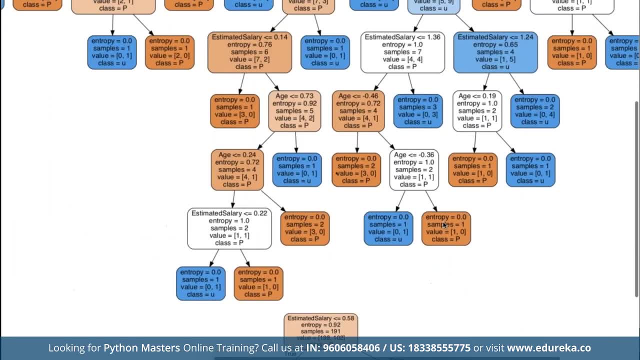 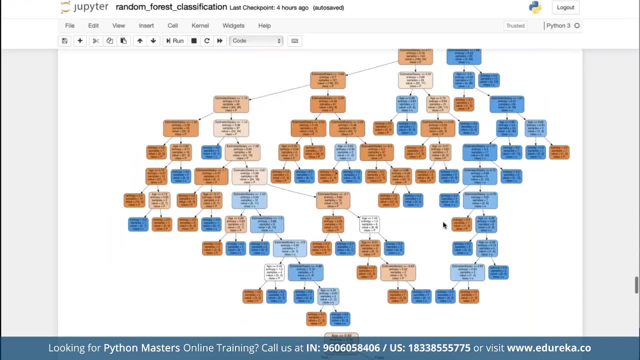 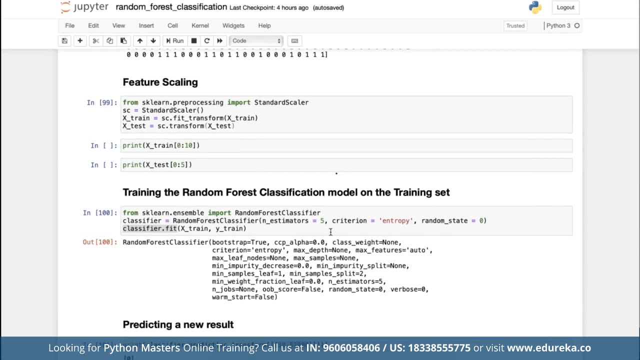 because they have taken this in at random. Now we just had two variables, right? If we have more variables and data will have to have like hundreds of trees, but you can do that all of that in your this model. So if I run it with five trees, 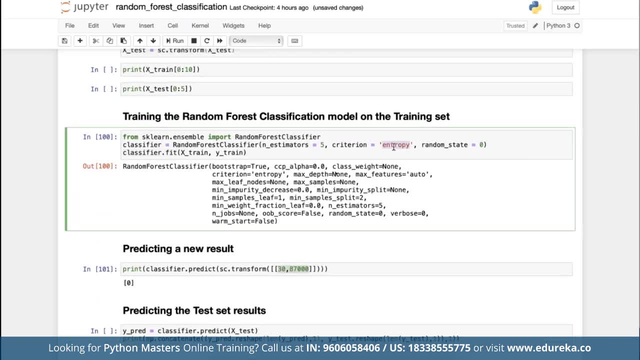 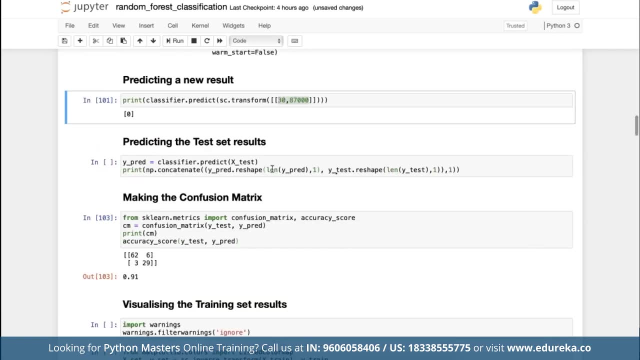 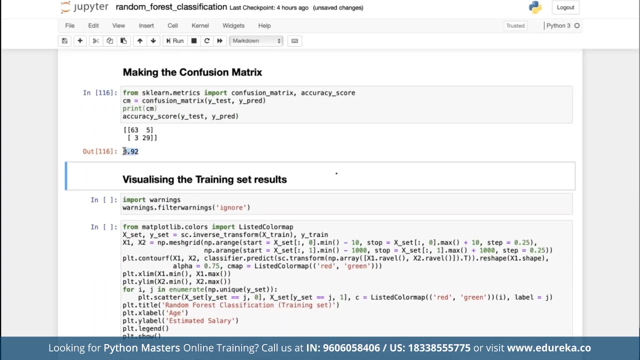 I am getting 91% accuracy. Let's quickly try to, for example, painting this with GD method for splitting and we don't change anything else, for example, and then, if we predict so, we have improved by one person. So this is how you will. 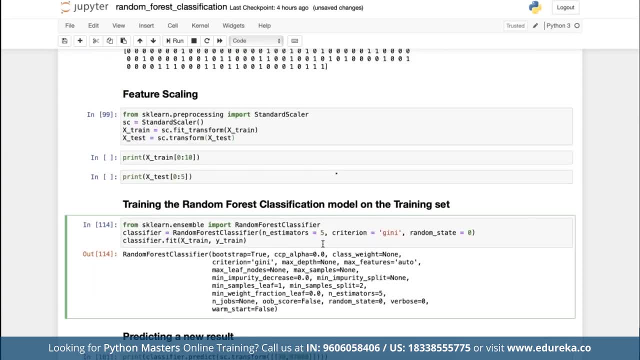 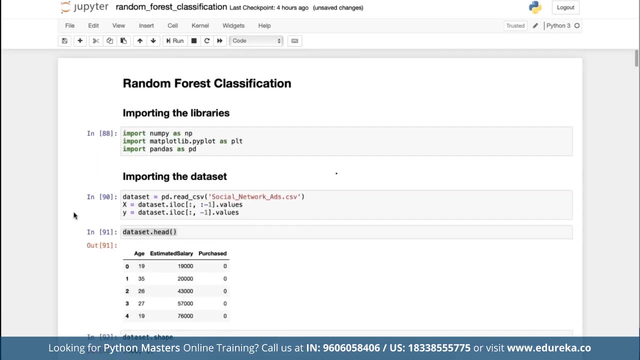 you know, keep tuning. using hyper meters You change this 5 to 10.. It might not change it because we just have two variables, but if there are more data, larger data sets, it would make a significant difference. So that's just one basic way of training. 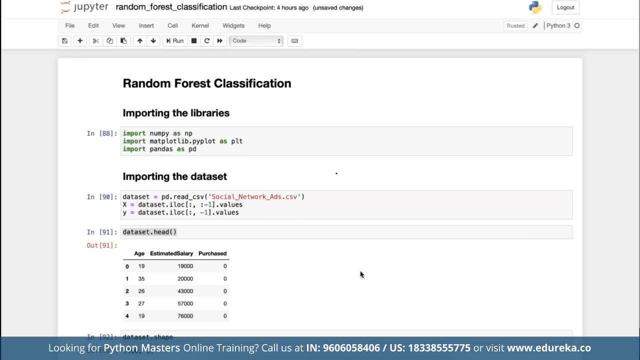 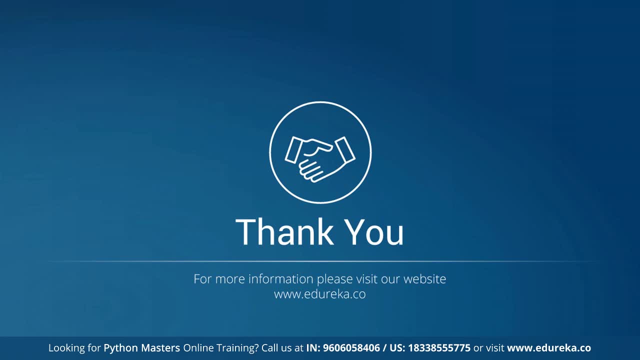 and seeing how it performs and how we can visualize the data. So I think we'll stop here. So I wish you all the best for your future learning and thank you for attending. Bye, Bye, Bye, Bye.